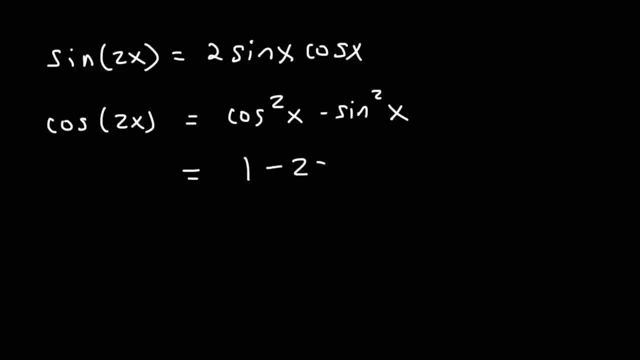 You can set it equal to 1 minus 2 sine squared Or 2 cosine squared minus 1.. Next up are the power reducing formulas. Sine squared can be reduced to 1 half 1 minus cosine 2x, And cosine 2x can be reduced to 1 half 1 minus cosine 2x. And cosine 2x can be reduced to 1 half 1 plus cosine 2x, And cosine 2x can be reduced to 1 half 1 minus cosine 2x, And then cosine squared can be reduced to 1 half 1 minus cosine 2x. 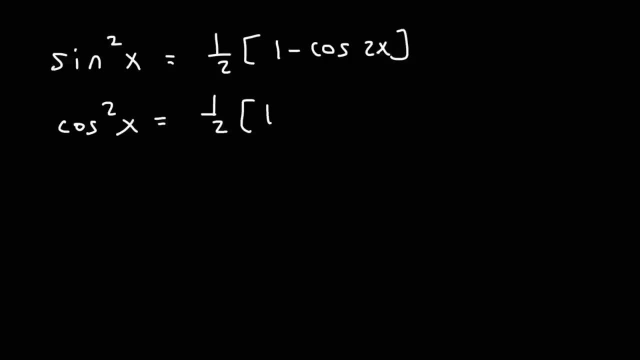 And cosine 2x can be reduced to 1 half 1 minus cosine 2x, And then cosine 2x can be reduced to 1 half 1 minus cosine 2x. Now there are some other trigonometric formulas that you may need to know, which I'll introduce later in this video when it becomes relevant. 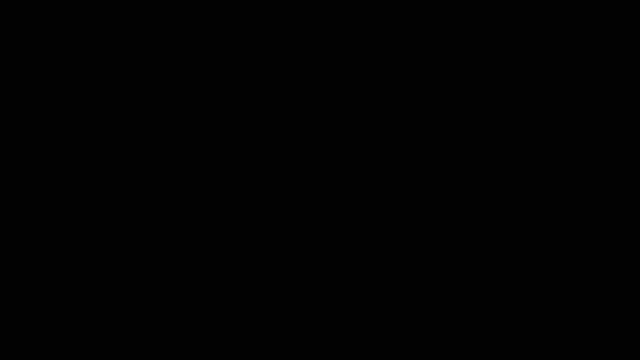 But for now, we can work with what we have here. Now, the first problem that we're going to work on is this one: Let's find the anti-derivative of cosine to the 3rd x. so what do you think we need to do here? what we could do is we can write cosine. 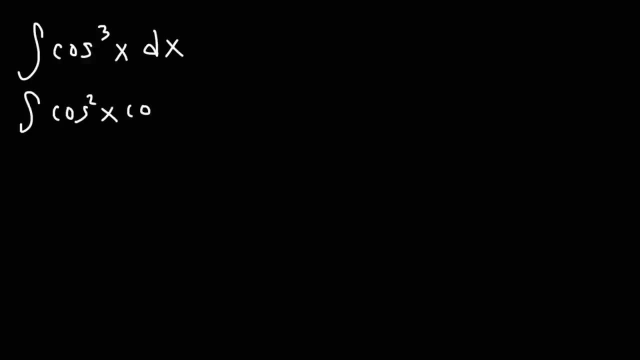 cube as cosine squared times cosine X, and what we want to do is we want to change cosine squared into 1 minus sine squared. keep in mind: sine squared plus cosine squared is equal to 1. solving for cosine, we can move sine squared to the other side. if we do that, we'll get that cosine squared is 1 minus sine squared. 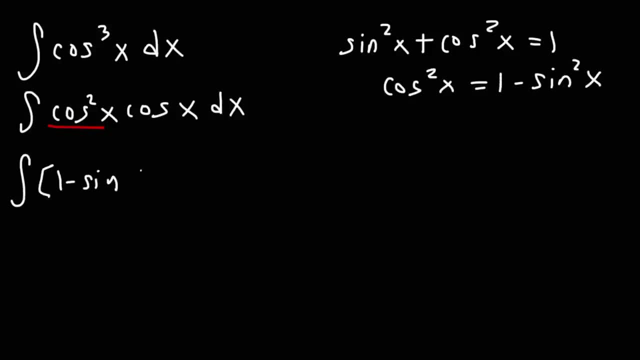 so we're going to replace cosine squared with 1 minus sine squared. now, the reason why we want to put it in this form is so that we can do u substitution. if we make u equal to sine X, D, u is going to be cosine X and x, so that's why we had to keep release one. 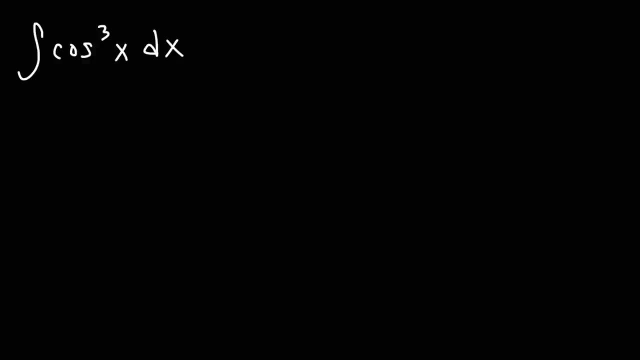 Let's try this one over here. so what do you think we need to do here? what we could do is we can write cosine cube as cosine squared times cosine X, and what we want to do is we want to change cosine squared into 1 minus sine squared. keep in mind: sine squared plus. 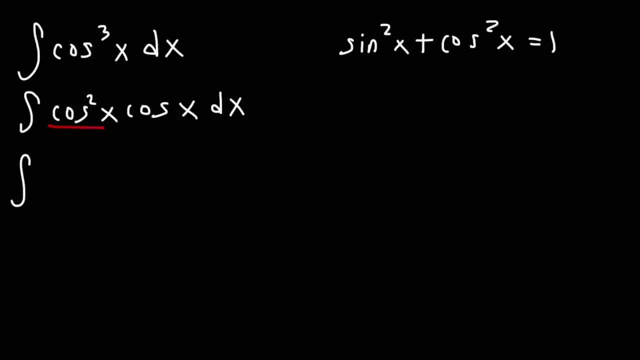 cosine squared is equal to 1, solving for cosine, we can move sine squared to the other side. if we do that, we'll get that cosine squared is 1 minus sine squared. so we're going to replace cosine squared with 1 minus sine squared. now the reason. 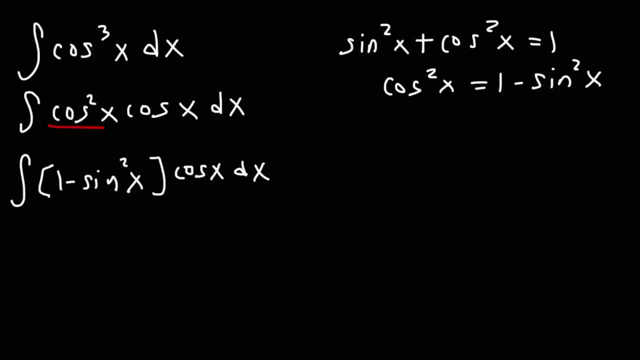 why we want to put it in this form is so that we can do u substitution. if we make u equal to sine X, D, u is going to be cosine X and DX. so that's why we have to keep at least one cosine on the outside, so that we can use it to change it into du. so this part. 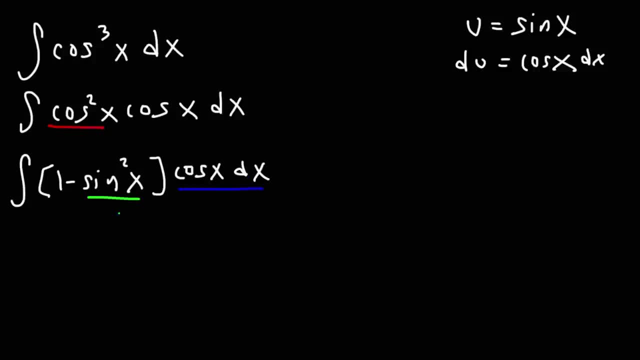 here is du, and we're going to replace sine with u, so this becomes the integral of 1 minus u squared du. the antiderivative of 1 is going to be u. the antiderivative of u is going to be sine, and we're going to replace sine with u. 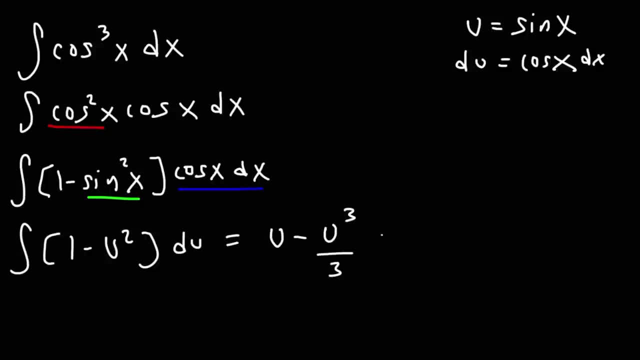 of u squared is u to the third over three and then plus c. Now our last step is to replace u with sine. So our final answer is going to be sine x minus one over three, sine to the third, x plus c. So that's the antiderivative of cosine cubed. 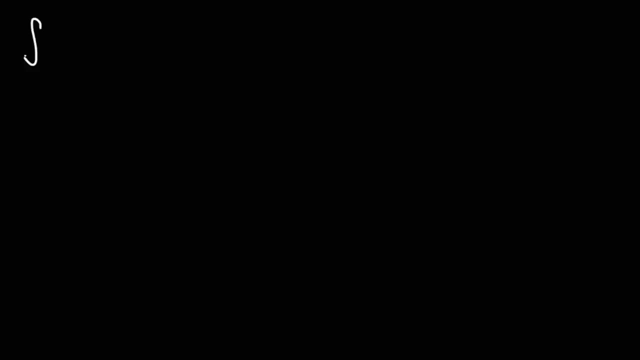 Now let's work on another similar problem, but one that's a little bit harder: Cosine raised to the fifth of x. Go ahead and find the antiderivative of that expression. So what we're going to do is we're going to take out a cosine. 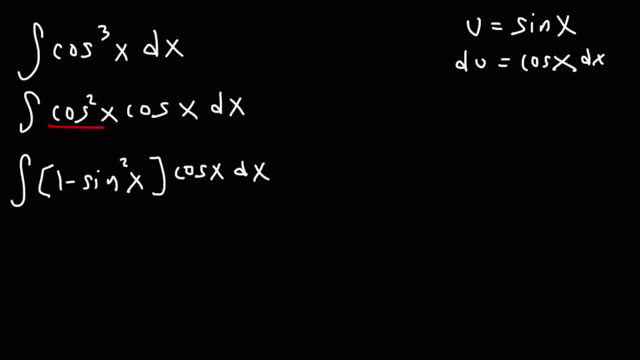 cosine on the outside so that we can use it to change it into of you. so this part here is due and we're going to replace sine with you. this becomes the integral of 1 minus u squared. DO, the anti-derivative of 1. it's going to be you, the anti-derivative of u. 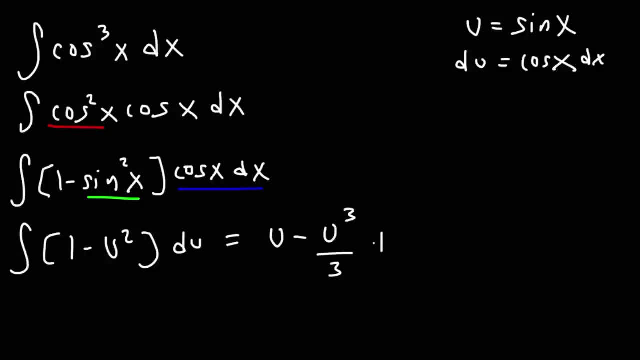 u squared is u to the third over 3, and then plus c. Now our last step is to replace u with sine. So our final answer is going to be sine x minus 1 over 3, sine to the third, x plus c. So that's the antiderivative of cosine cubed. Now let's work on another similar. 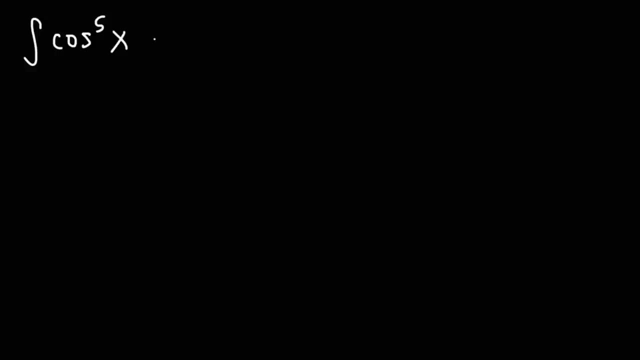 problem, but one that's a little bit harder. Cosine raised to the fifth of x. Go ahead and find the antiderivative of that expression. So what we're going to do is we're going to take out a cosine, So this is going to be cosine to the fourth times, cosine x, dx. Now, 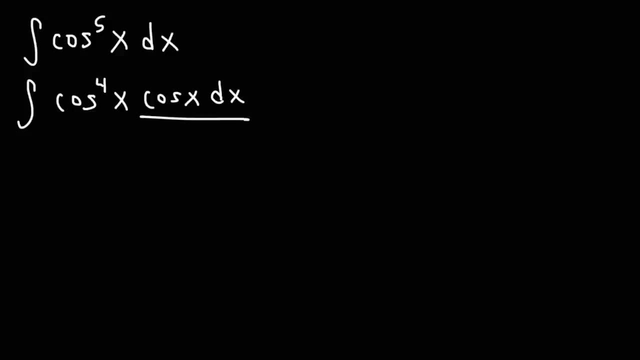 we want this to become eventually du, like we did before. So we need to change cosine into sine, But we need to get cosine squared first. Cosine to the fourth is cosine squared squared. Now cosine squared, we can make that 1 minus sine squared. 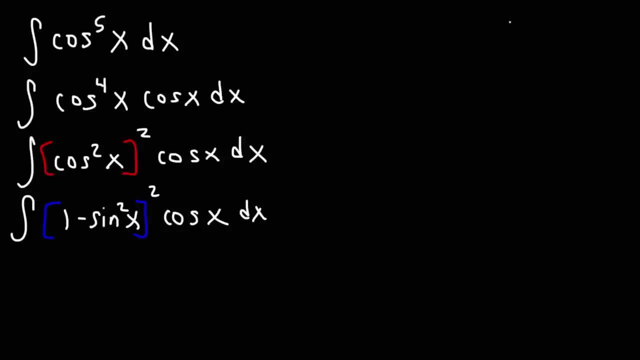 Now, at this point we can replace sine squared with cosine squared, So we're going to replace sine with u. du is going to be cosine x- dx, So we're going to replace this with du. So this becomes the integral of 1 minus u squared, raised to the. 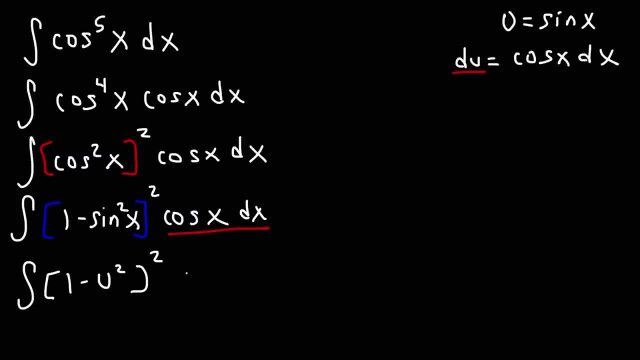 second power, And all of this can be replaced with du. Now, before we can integrate this expression, we need to expand it. So what we have is 1 minus u squared times 1 minus u squared, So let's FOIL 1 times. 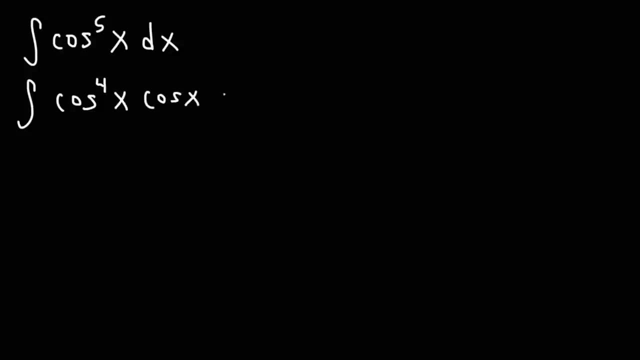 So this is going to be cosine to the fourth times, cosine x, dx. Now we want this to become a variable, do you like we did before. so we need to change cosine into sine, but we need to get cosine squared first. cosine to the fourth is cosine squared- squared now. 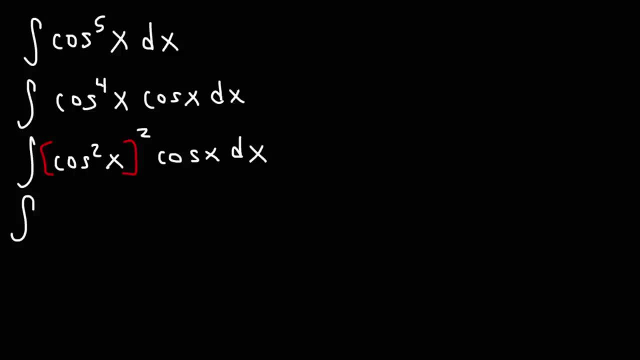 cosine squared. we can make that 1 minus sine squared now. at this point we can replace sine with u. du is going to be cosine x, dx, so we're going to replace this with du. so this becomes the integral of 1 minus u squared raised to the second power, and all of this can be replaced with du now. 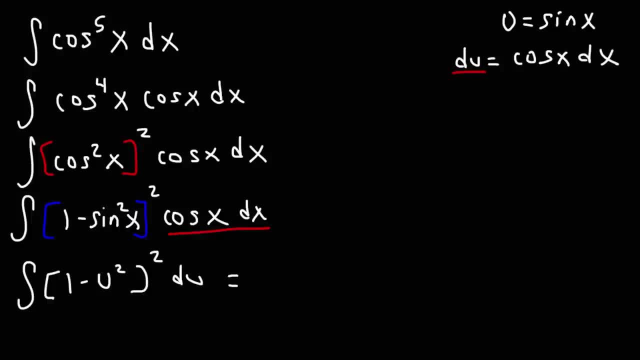 my. before we can integrate this expression, we need to expand it. so what we have is 1 minus u squared times 1 minus u squared. so let's foil 1 times 1 and that's going to be 1, and then this is negative u squared plus another negative. 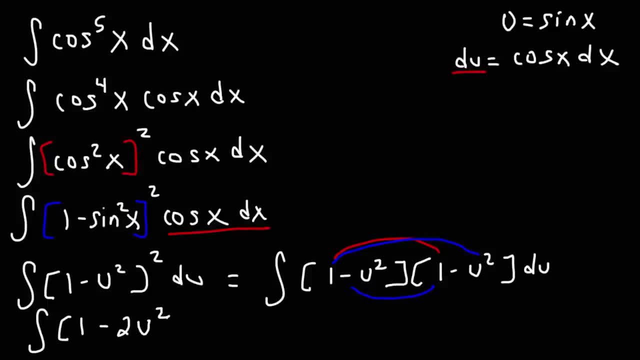 u squared, so that's going to be negative 2 u squared, and then negative u squared. times negative u squared, that's going to be positive u to the fourth, and then times du. so now let's go ahead and find the anti derivative of this expression, so it's: 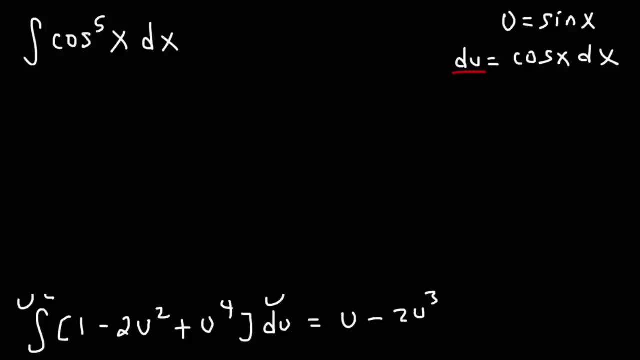 going to be you minus 2u to the third over 3, plus u to the fifth power over 3, plus u to the 5th power over 5, using the power rule and then plus the constant of integration. So now we can write our final answer. 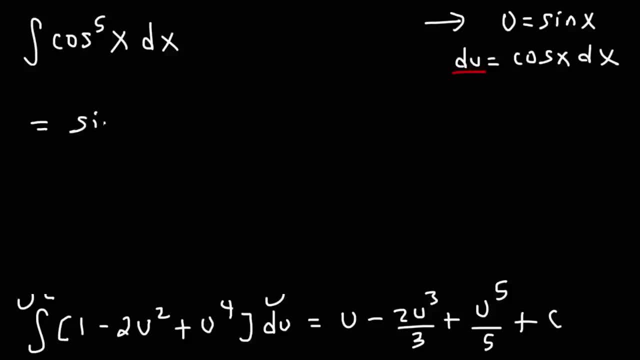 Let's replace u with sine, So we're going to have sine x minus 2 over 3, sine to the 3rd power of x, and then plus 1 over 5, sine to the 5th power of x plus c. 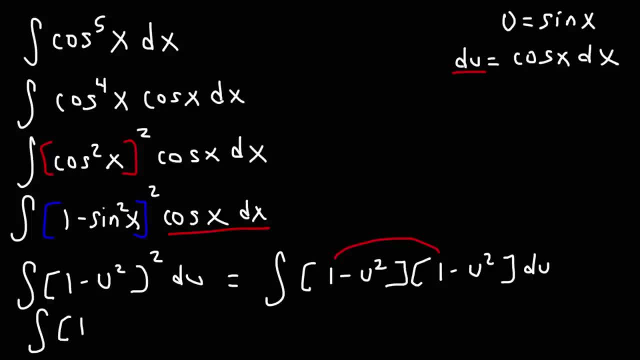 1.. And that's going to be 1.. And then this is negative u squared plus another negative u squared, So that's going to be negative 2 u squared. And then negative u squared times negative u squared, That's going to be positive u to the fourth, And then this: 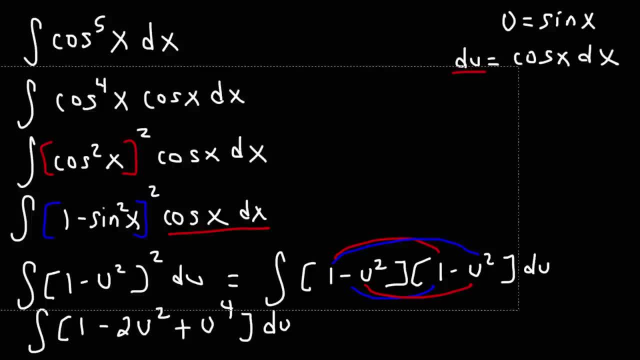 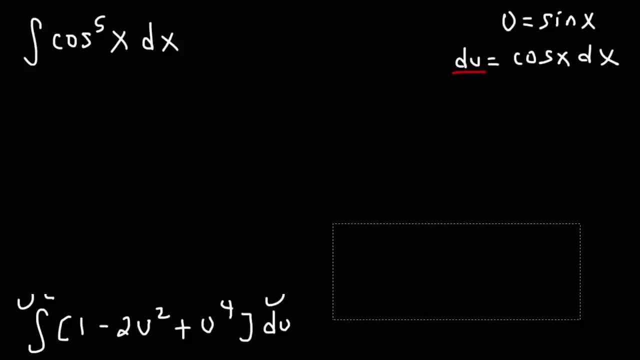 is negative, 2, u squared, And then times du. So now let's go ahead and find the antiderivative of this expression. So it's going to be u minus 2, u to the third over 3, plus u to the fifth, power over 5, using the power rule, And. 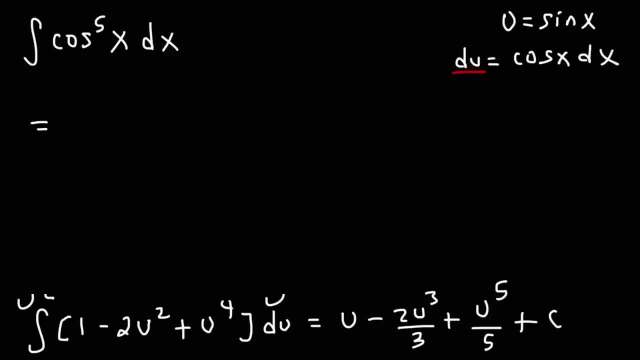 then plus the constant of integration. So now we can write our final answer. Let's replace u with sine. So we're going to have sine x minus 2 over 3, sine to the third power of x and then plus 1 over 5, sine to the fifth power of x plus c. 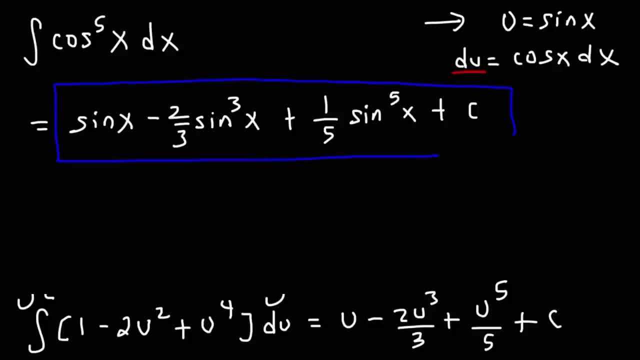 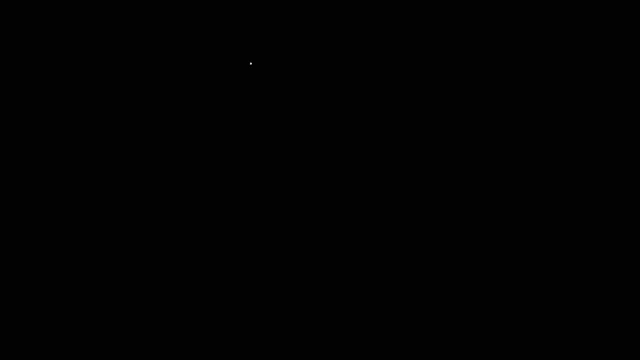 So this is the indefinite integral of cosine x raised to the fifth power. So this is our final answer. Now let's try another problem. Let's find the indefinite integral of cosine to the fifth x times sine x dx. Feel free to try this problem. 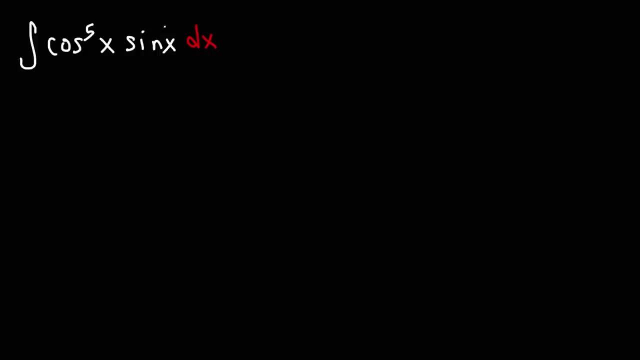 So what should we do here? Notice that we have a sine by itself. So what we want to do is we want to make u equal to cosine, Because du is going to have the sine that we need. So we need to cancel this sine. 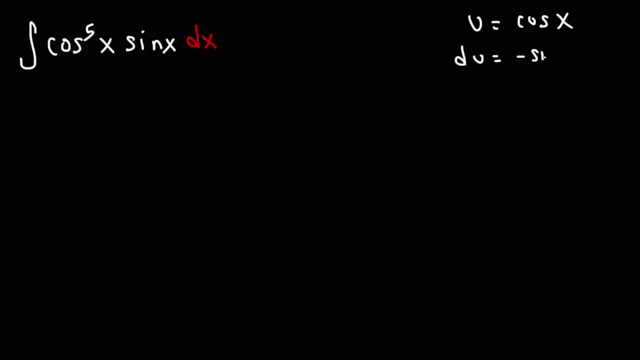 The derivative of cosine is negative sine And if we solve for dx it's going to be du divided by negative sine. So we can go ahead and replace cosine with u, So this will be u to the fifth power, And then we can replace dx with what we have here. 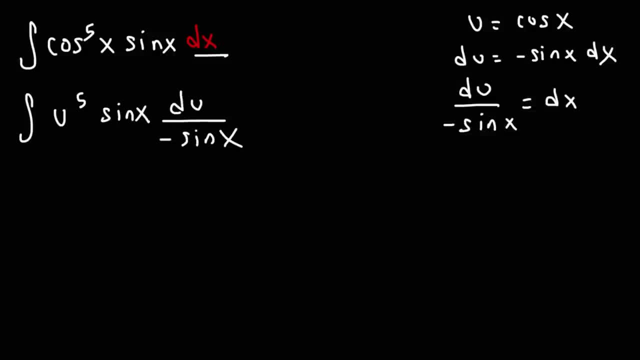 du over negative sine x, Sine will cancel. So we're going to have the integral of negative u to the fifth du And then, using the power rule, it's going to be negative u to the sixth over 6 and then plus c. 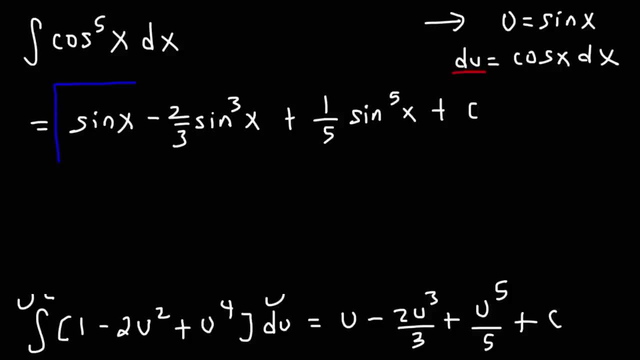 So this is the indefinite integral of cosine x raised to the 5th power. So this is our final answer. Now let's try another problem. Let's find the indefinite integral of cosine to the 5th x times sine x dx. Feel free to try this problem. 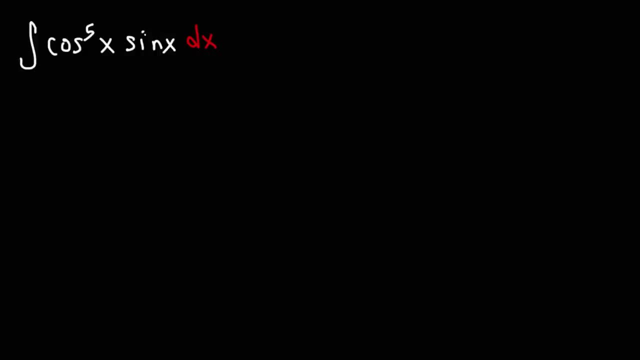 So what should we do here? Notice that we have a sine by itself. So what we want to do is we want to make u equal to cosine, because du is going to have the sine that we need to cancel this sine. The derivative of cosine is negative sine. 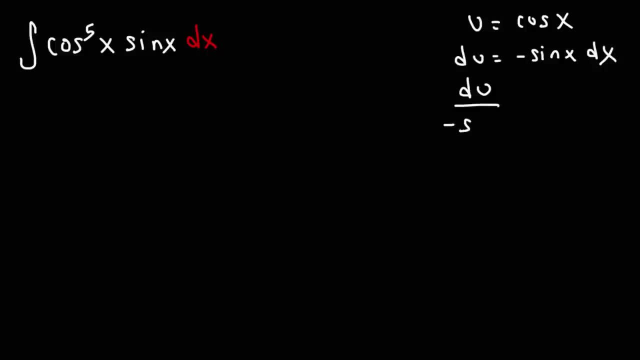 And if we solve for dx, it's going to be du divided by negative sine. So we can go ahead and replace cosine with u, So this will be u to the 5th power, And then we can replace dx with what we have here. 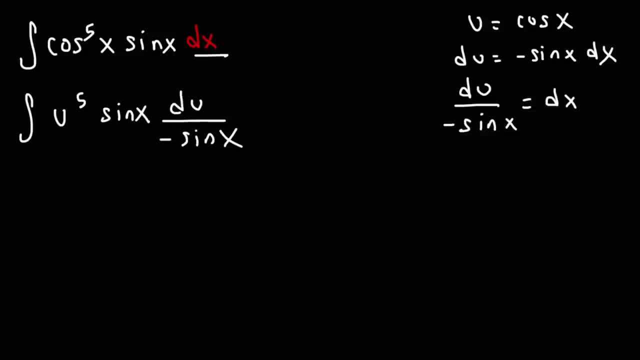 du over negative sine x Sine will cancel. So we're going to have the integral of negative u to the 5th du and then, using the power rule, it's going to be negative u to the 6th over 6th. 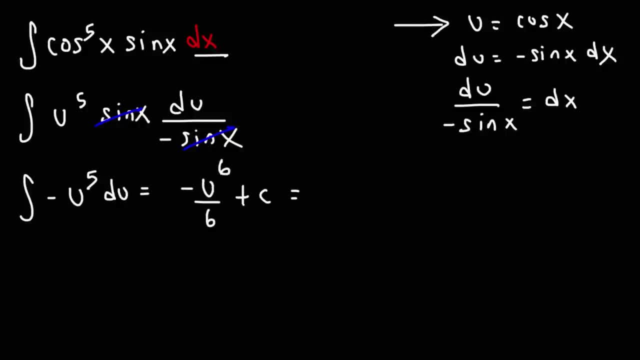 and then plus c. So now we've just got to replace u with cosine, And so our final answer is going to be negative: 1 over 6 cosine to the 6th power of x plus c. So this is the answer. 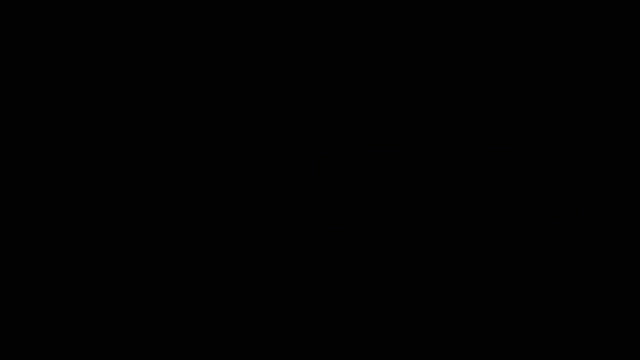 This problem wasn't too bad. It was pretty straightforward. Now let's try a similar problem that is going to be a little bit longer than the other one. So let's find the indefinite integral of sine to the 5th power times, cosine squared of x, dx. 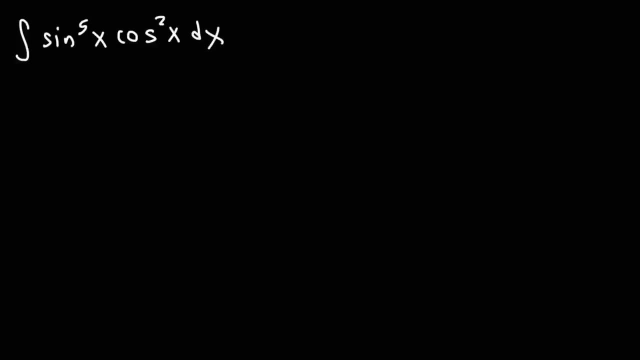 Feel free to pause the video If you want to. Now the question is: should we make u equal to sine or cosine? Cosine has an even power, Sine has an odd power. What we want to do is we want to make u equal to cosine. 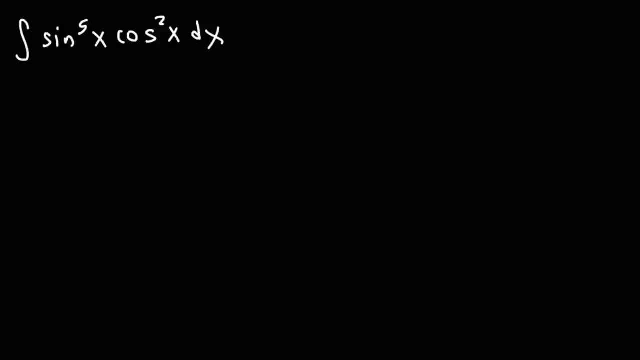 Because what we could do is take out a sine, leave it by itself and then the sine to the 4th. we can convert all of that into cosine. So let me show you Sine to the 5th. we're going to write that as: 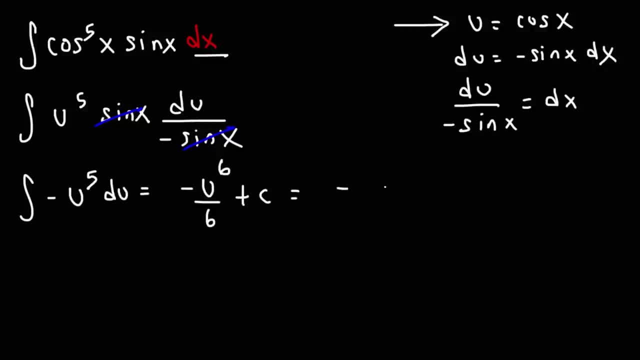 So now we just got to replace u with cosine, And so our final answer is going to be negative: 1 over 6: cosine to the sixth power of x plus c. So this is the answer. This problem wasn't too bad, It was pretty straightforward. 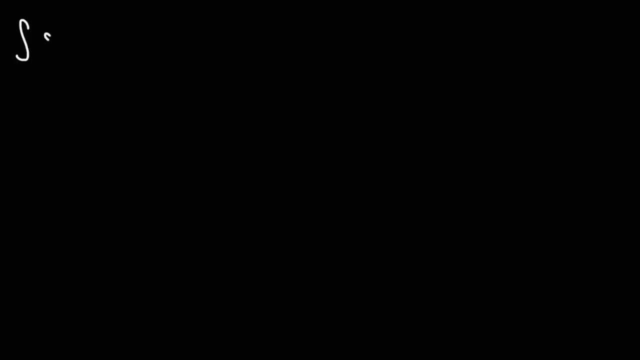 Now let's try a similar problem. that is going to be a little bit longer than the other one. So let's find the indefinite integral of sine to the fifth power times: cosine squared of x- dx. Feel free to pause the video if you want to. 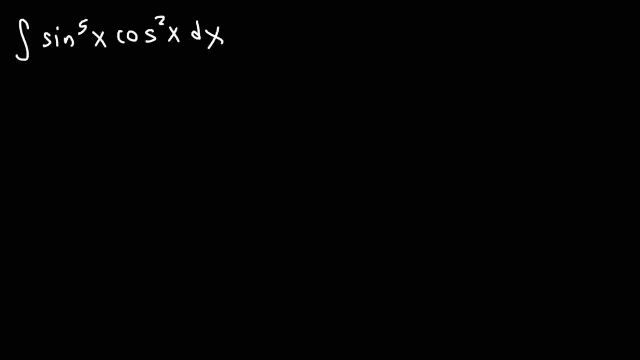 Now the question is: should we make u equal to sine or cosine? Cosine has an even power, Sine has an odd power. What we want to do is we want to make u equal to cosine, Because what we could do is take out a sine, leave it by itself, and then the sine to the fourth. we can convert all of that into cosine. 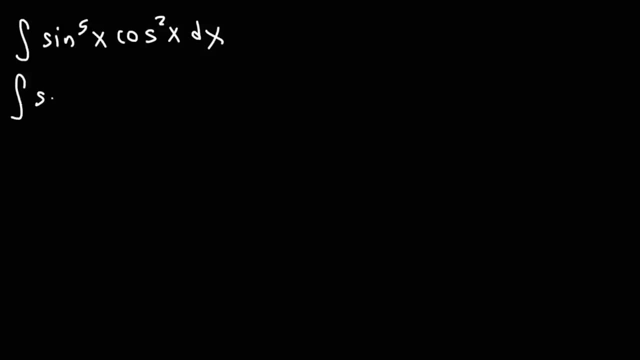 So let me show you Sine to the fifth. we're going to write that as sine. to the fourth: x times sine, times cosine squared This sine. We want that to pair up with the dx, because that's going to be our du. 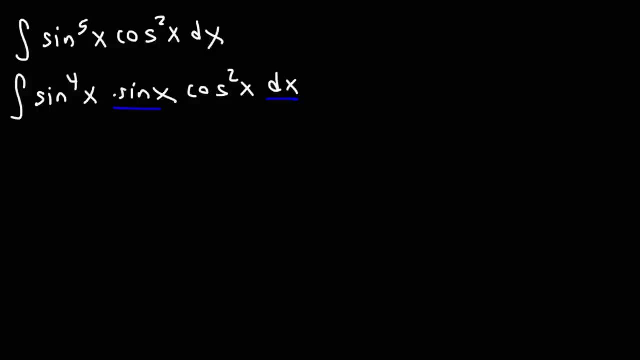 Everything else we want it to be not in terms of sine, but cosine Sine. to the fourth, I'm going to write that as sine squared, squared, And then we have cosine squared and I'm going to put sine next to dx. 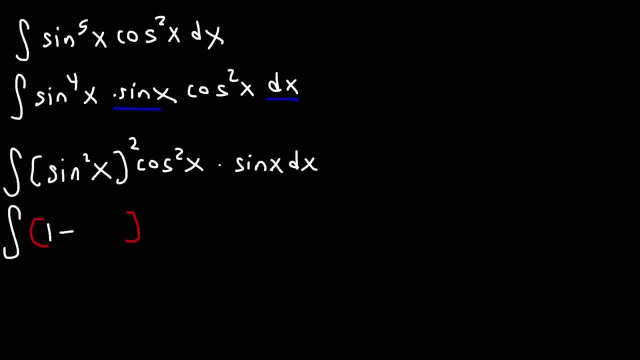 Now we know that sine squared is 1 minus cosine squared, Based on the trig identity, sine squared plus cosine squared is 1.. And now we have everything in terms of cosine, except this particular trig function, sine. So now we can make u equal to cosine. 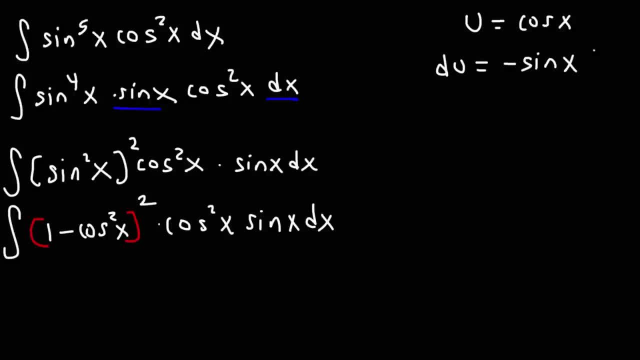 du is going to be negative. sine x, dx. So dx is this. So everywhere we see a cosine, we're going to replace it with u. So this is going to be 1 minus u squared squared times u squared times sine x. 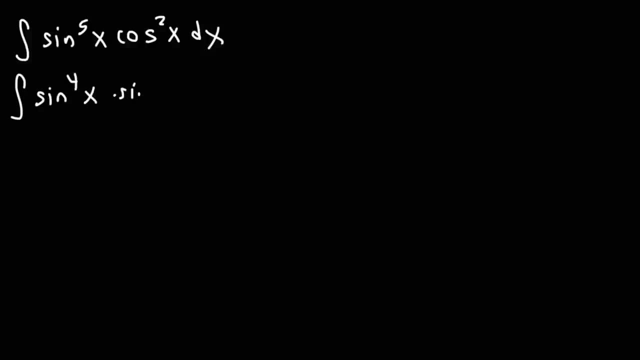 sine to the 4th. x times sine, times cosine squared This sine. we want that to pair up with the dx, because that's going to be our du. Everything else, we want it to be not in terms of sine but cosine. 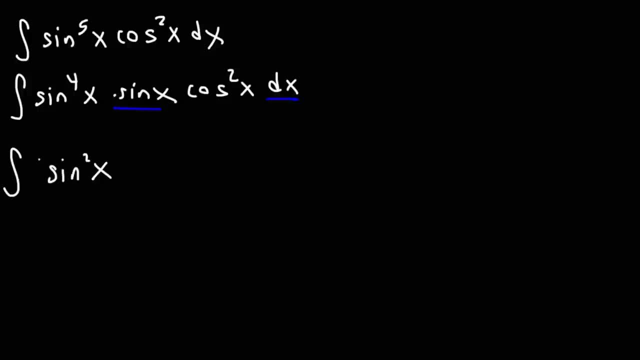 Sine to the 4th. I'm going to write that as sine squared squared. And then we have- and I'm going to put sine next to dx. Now we know that sine squared is 1 minus cosine squared, Based on the trig identity. 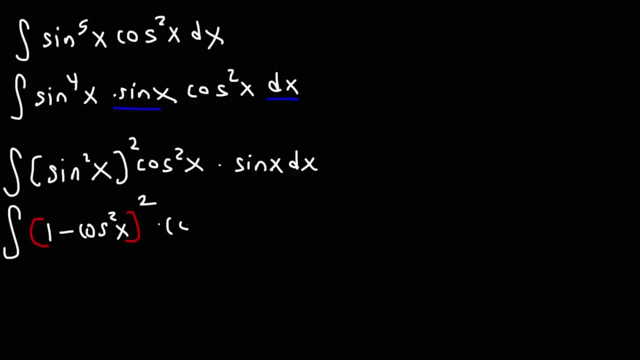 sine squared plus cosine squared is 1.. And now we have everything in terms of cosine except this particular trig, function, sine. So now we can make u equal to cosine And du is going to be negative sine, x, dx. So dx is this: 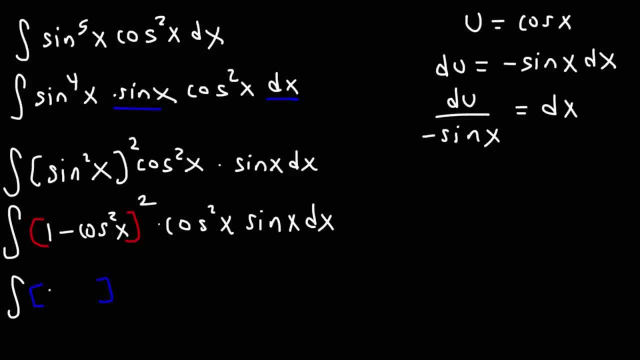 So everywhere we see a cosine, we're going to replace it with u. So this is going to be 1 minus u squared squared times u, squared times sine x. And then let's replace dx with du, with u, du over negative sine x. 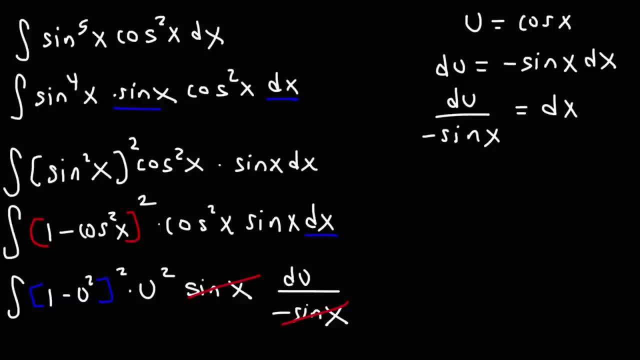 So these will cancel, And what we need to do next is we need to FOIL. So this is what we have at this point, And let's not forget the negative sine that we have here, So I'm going to put that in the front. 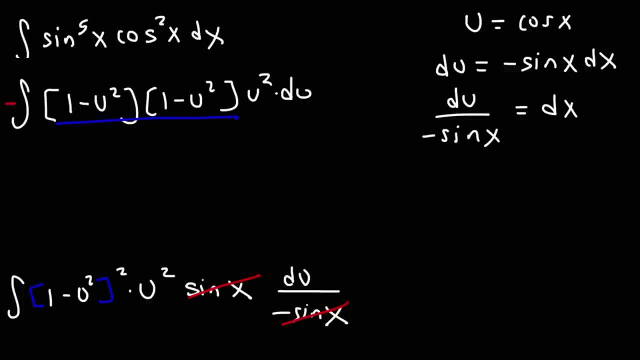 Now we've already FOILed 1 minus u squared times: 1 minus u squared. Based on a previous problem, we know it's going to be 1 minus 2u squared plus u to the 4th. Our next step is to distribute u squared. 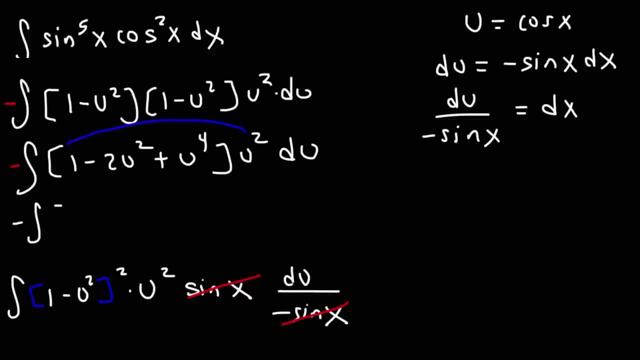 So u squared times 1, that's going to be u squared. But let's go ahead and distribute this negative sine as well, So it's going to be negative. u squared. And then u squared times negative. 2u squared times the negative sine. 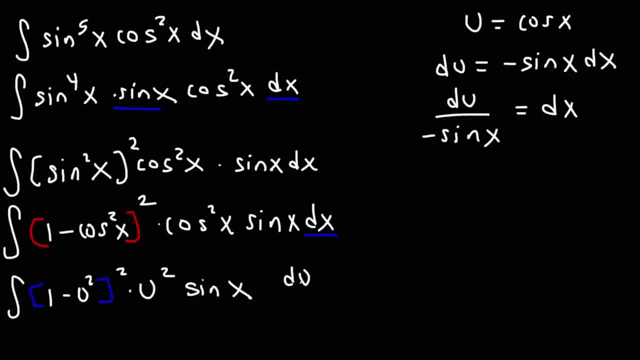 And then let's replace dx with du over negative sine x. So these will cancel, And what we need to do next is we need to FOIL. So this is what we have at this point, And let's not forget the negative sine that we have here. 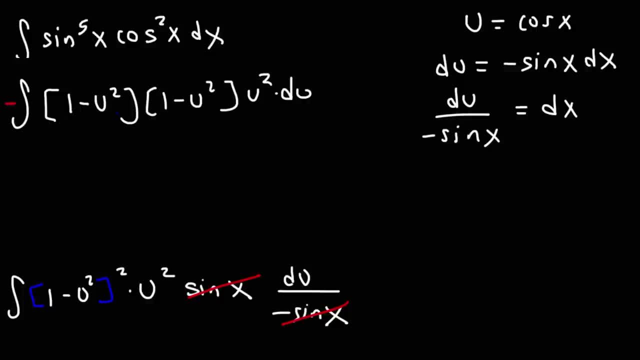 So I'm going to put that in the front Now. we've already FOILed 1 minus u squared times 1 minus u squared. Based on a previous problem, we know it's going to be 1 minus 2u squared plus u to the fourth. Our next step is to distribute u squared. 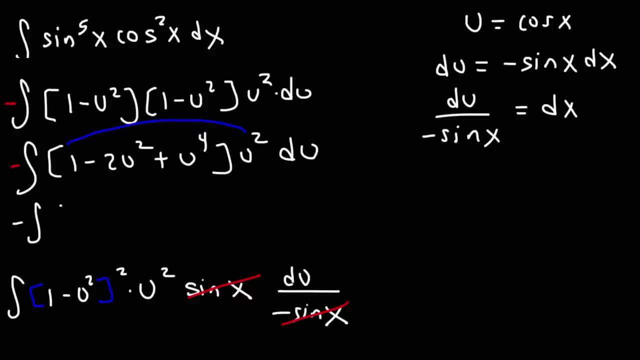 So u squared times 1, that's going to be u squared. But let's go ahead and distribute this negative sign as well. So it's going to be negative. u squared, And then u squared times negative. 2u squared times- the negative sign. that's going to be positive. 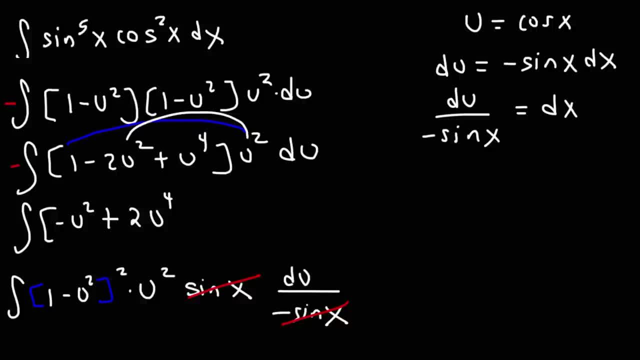 2u to the fourth, And then u squared times u to the fourth with the negative in front, that's going to be negative u to the sixth. So now let's go ahead and find the antiderivative of each of these terms. So it's going to be: 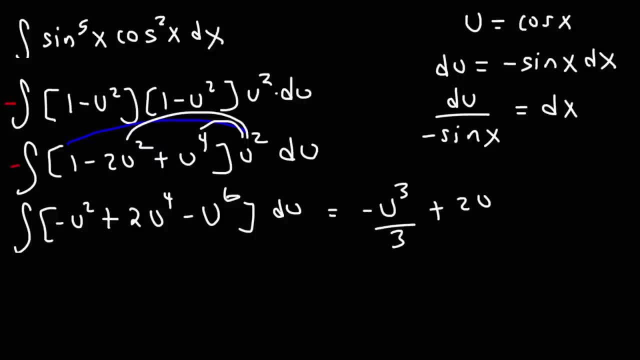 negative: u to the third over 3 plus 2u to the fifth over 5, minus u to the seventh over 7 plus c. So now let's go ahead and replace u with cosine, So it's going to be negative 1 over 3 cosine to the third power plus 2 over 5. 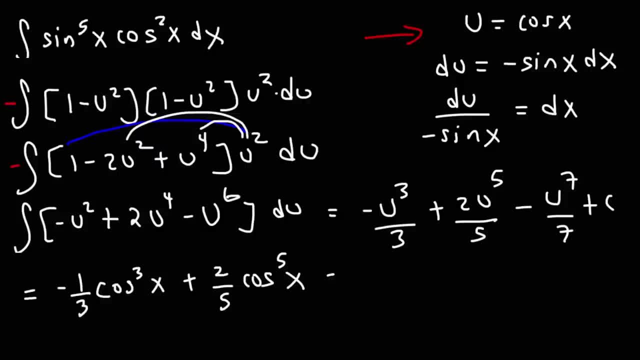 cosine to the fifth power minus 1 over 7. cosine to the seventh power plus c. So this right here is going to be our final answer. So that is the antiderivative of sine to the fifth, x to the fifth. So now let's go ahead and find the antiderivative of sine to the fifth power of x times cosine squared x. 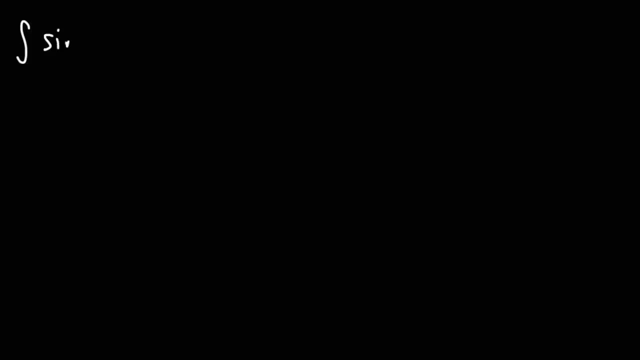 Here's another similar problem. Let's find the indefinite integral of sine to the fifth power of x times cosine cubed x. Try that one. Now we got to decide if we want to make u equal to sine or cosine, Because we can isolate a sine from the integral. 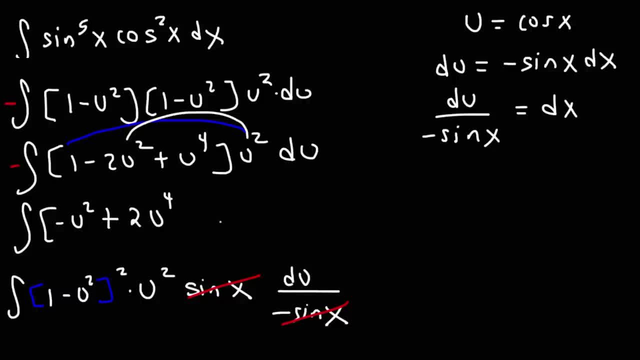 That's going to be positive. 2u to the 4th. And then u squared: times: u to the 4th with the negative in front. That's going to be negative. u to the 6th. So now let's go ahead and find. 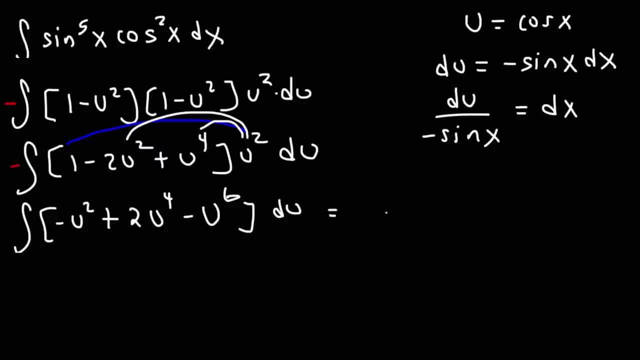 the antiderivative of each of these terms. So it's going to be negative: u to the 3rd over 3.. Plus: 2u to the 5th over 5.. Minus: u to the 7th over 7.. 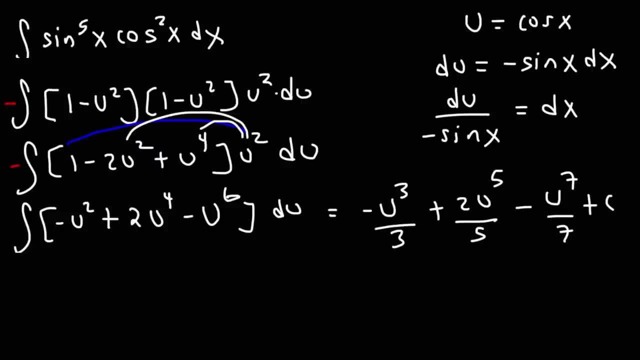 Plus c. So now let's go ahead and replace u with cosine, So it's going to be negative 1 over 3. Cosine to the 3rd power Plus 2 over 5. Cosine to the 5th power. 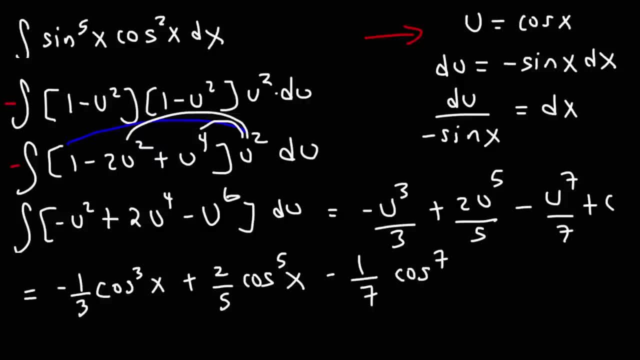 Minus 1 over 7.. Cosine to the 7th power Plus c. So this right here is going to be our final answer. So that is the antiderivative of sine to the 5th x times cosine squared x. 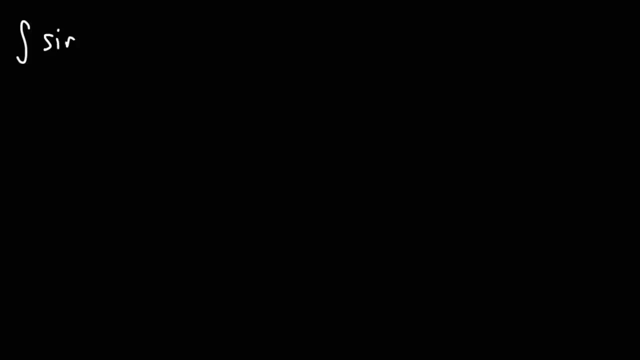 Here's another similar problem. Let's find the indefinite integral of sine to the 5th power of x times cosine cubed x. Try that one. Now we've got to decide if we want to make u's equal to sine or cosine. 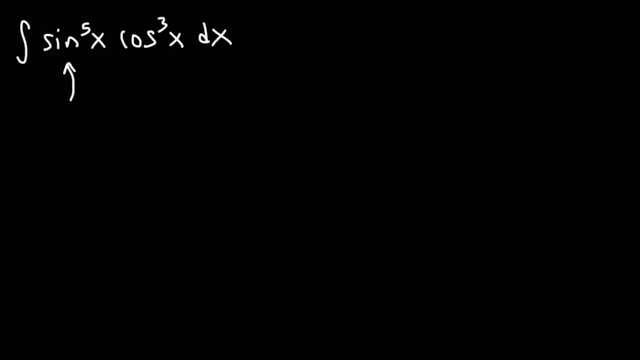 Because we can isolate a sine from the integral. We can split that into sine to the 4th x sine. Or we can split this into cosine squared x cosine. I think it's easier if we split cosine cubed into cosine squared x cosine. 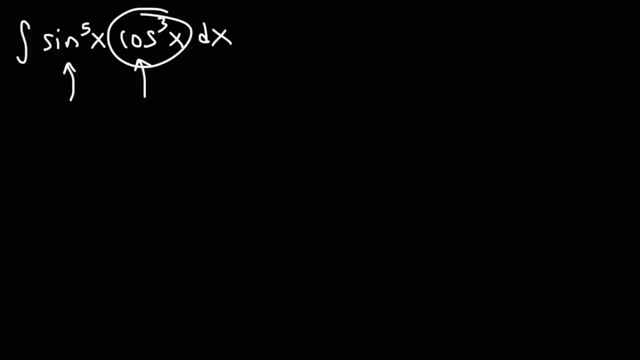 And then convert the cosine squared into 1 minus sine squared, Leaving that last cosine to be with dx. Let's do it that way Because to change this to sine to the 4th times sine, And then to convert sine to the 4th into. 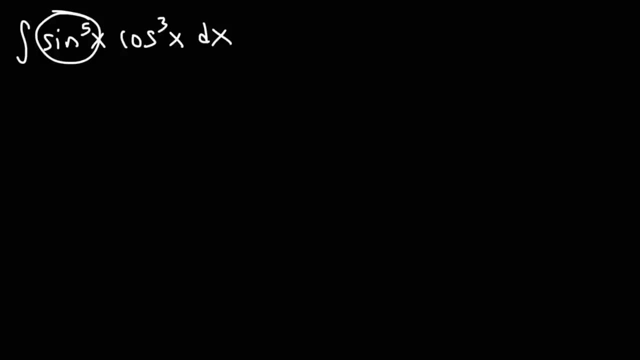 sine squared, times sine squared. That's going to be more work If we focus on this one, If we split it apart, And since it's easier to deal with 3 than 5. We don't have to FOIL, So it's easier if we. 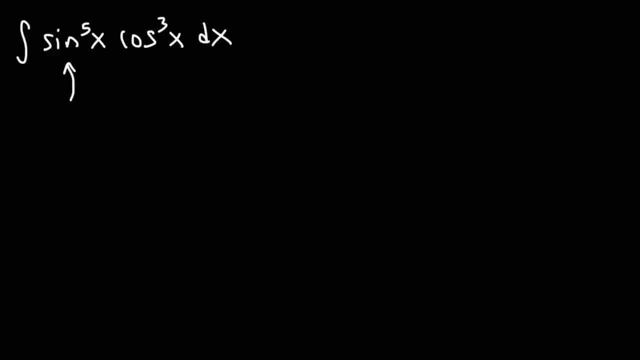 We can split that into sine to the fourth times sine, Or we could split this into cosine squared times cosine. I think it's easier if we split cosine cubed into cosine squared times cosine And then convert the cosine squared into 1 minus sine squared. 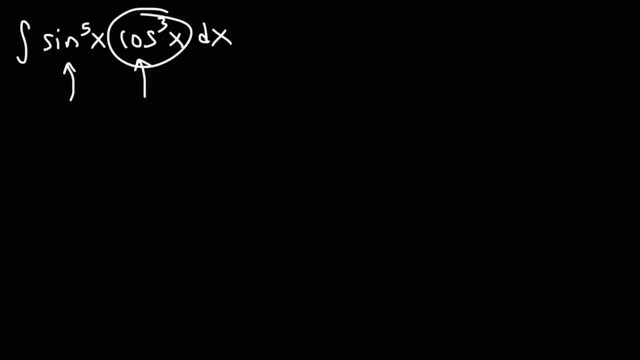 Leaving that last cosine to be with dx. Let's do it that way, Because to change this to sine, to the fourth times sine, And then to convert sine to the fourth into sine squared times sine squared, That's going to be more work. 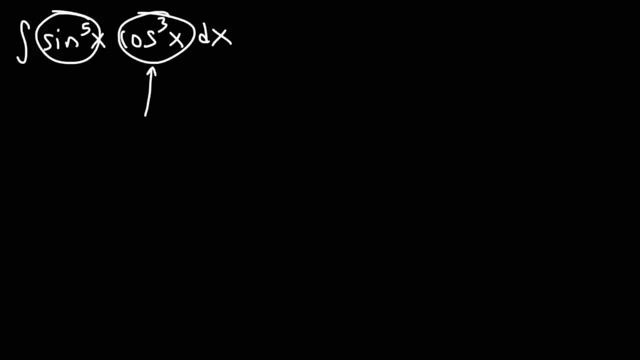 If we focus on this one, If we split it apart, And since it's easier to deal with 3 than 5. We don't have to FOIL. So it's easier if we break up cosine cubed into cosine squared and cosine. 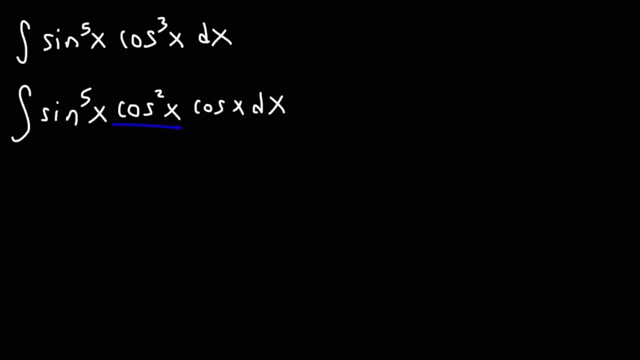 Now all we need to do is change cosine squared into 1 minus sine squared. So now we have everything in terms of sine, Except one cosine function. So now let's go ahead and make u equal to sine x, And du will simply be cosine x- dx. 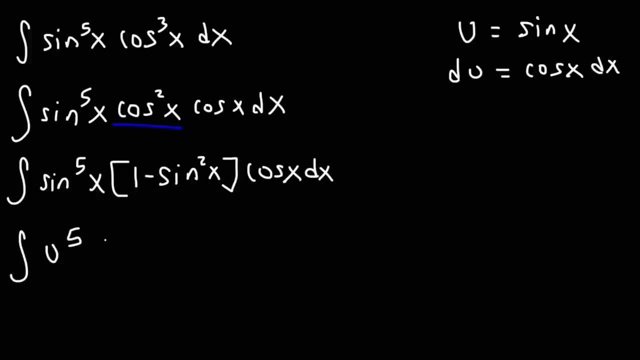 So this is going to be u to the fifth, And then we're going to make u to the fifth And then times 1 minus u squared, And then cosine x- dx. We could simply replace that with du. Now let's distribute the u to the fifth to 1 minus u squared. 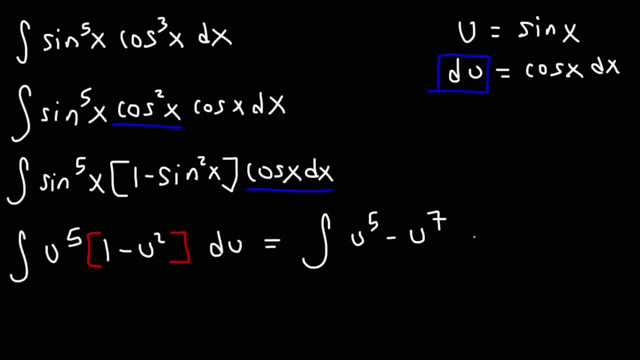 So it's going to be u to the 5 minus u to the 7.. And then du. The antiderivative of u to the 5 is going to be u to the 6 over 6. And then, for u to the 7th, that becomes u to the 8 over 8.. 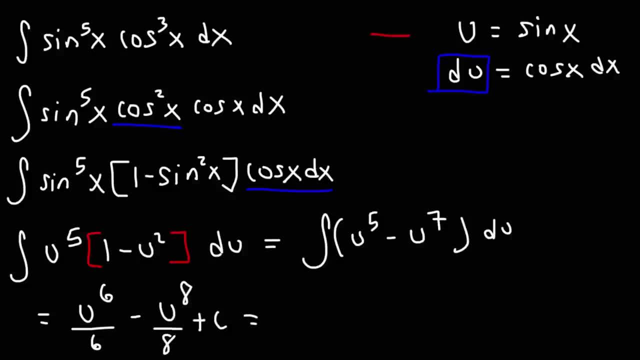 Plus c. Now let's replace u with sine x, So the final answer is going to be 1 over 6.. Sine to the 6th power: of x Minus 1 over 8. Sine to the 8: x plus c. 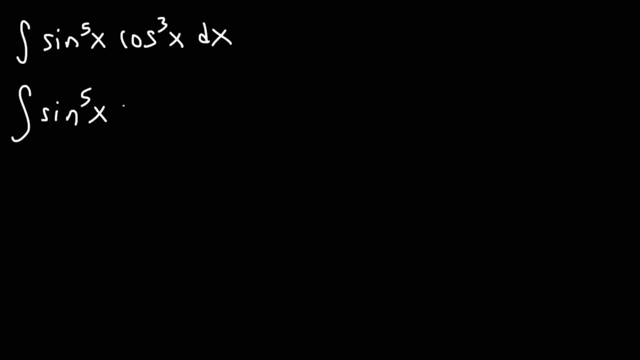 break up cosine cubed into cosine squared And cosine. Now all we need to do is change cosine squared into 1 minus sine squared. So now we have everything in terms of sine Except one cosine function. So now let's go ahead and make u. 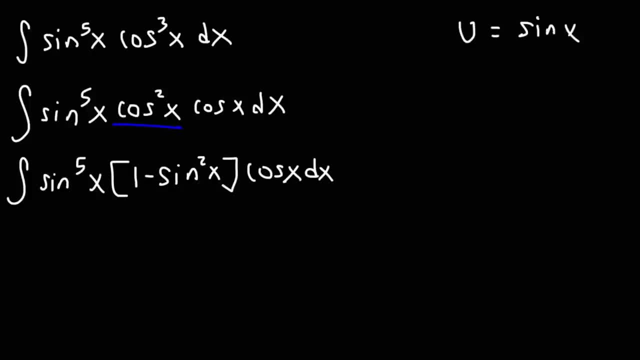 equal to sine x, And du will simply be cosine x- dx. So this is going to be u to the 5th, And then times 1 minus u squared, And then cosine x- dx. We could simply replace that with du. Now let's distribute the u to the 5th. 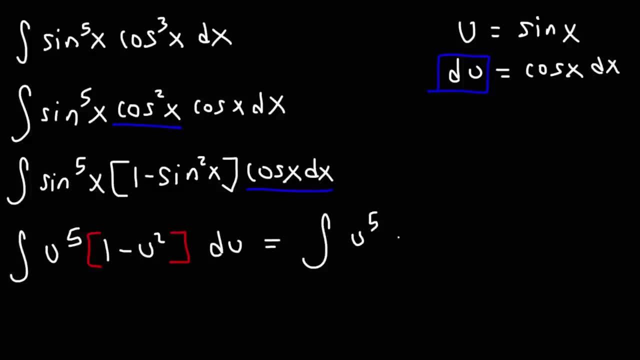 to 1 minus u squared. So it's going to be u to the 5 minus u to the 7.. And then du, The antiderivative of u to the 5 is going to be u to the 6 over 6.. And then for. 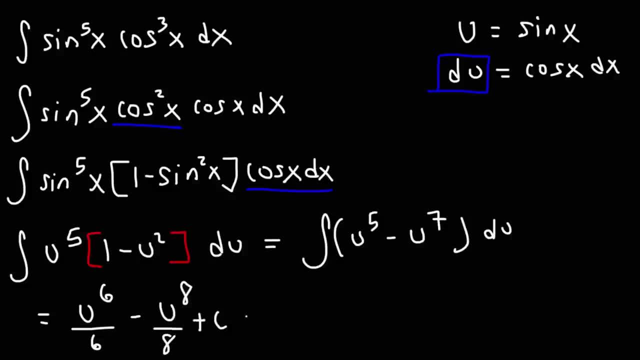 u to the 7th, that becomes u to the 8 over 8 plus c. Now let's replace u with sine x, So the final answer is going to be 1 over 6. sine to the 6th, power of x minus. 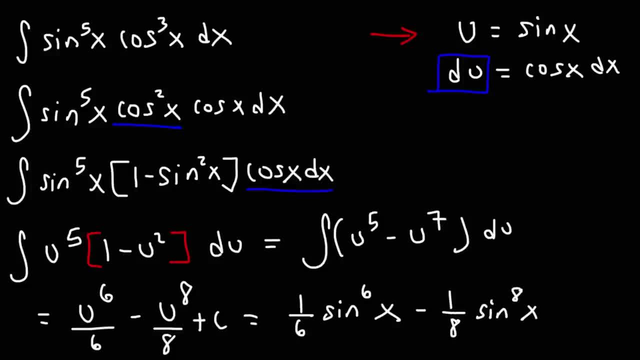 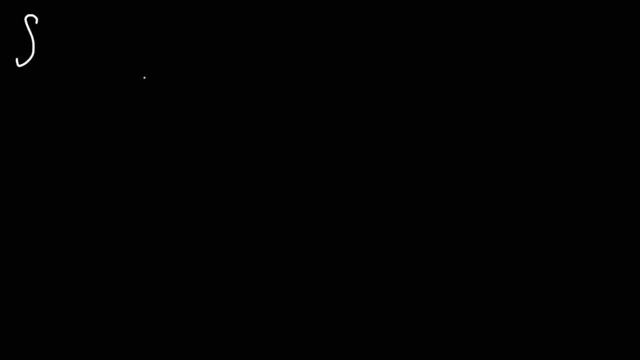 1 over 8 sine to the 8 x plus c. So this is the indefinite integral of the original problem. Now the next problem that we need to work on is finding the indefinite integral of sine squared x. Now this problem is definitely different from. 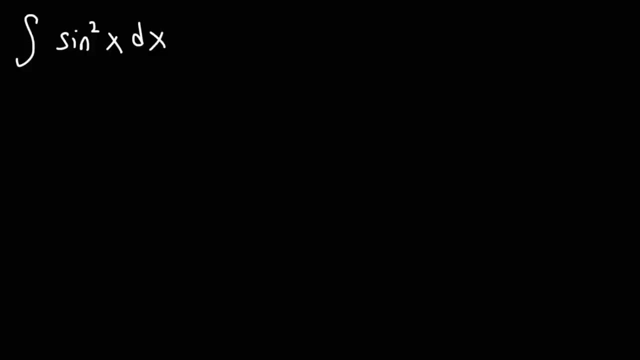 what we've been doing before. So what do you recommend that we should do here? Because it's not really advantageous to convert this into 1 minus cosine squared. In this case, we need to use the power reducing formulas. If you recall, earlier at the beginning of the video, we wrote that 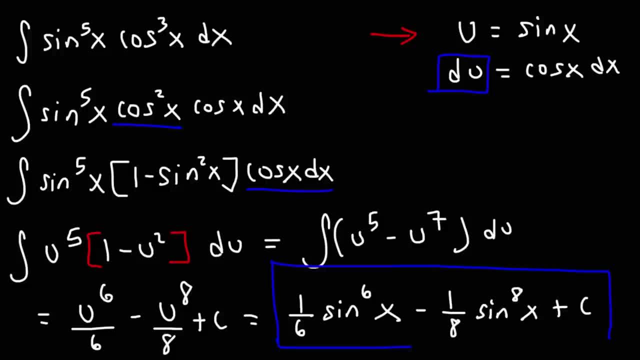 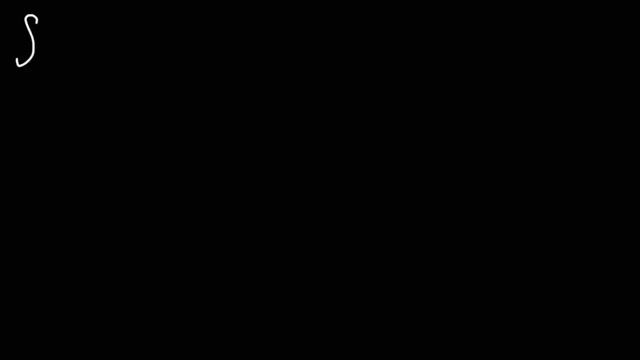 So this is the indefinite integral Of the original problem. Now the next problem that we need to work on Is finding the indefinite integral of sine squared x. Now this problem is definitely different from what we've been doing before, So what do you recommend that we should do here? 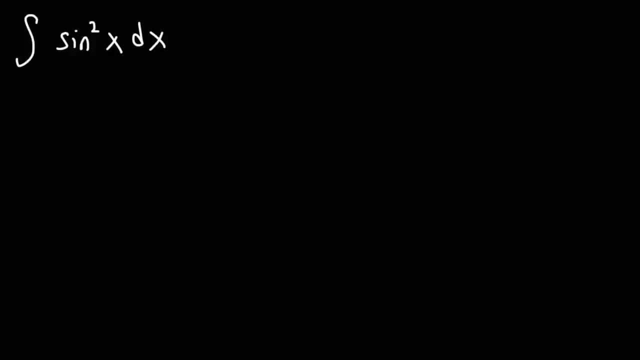 Because it's not really advantageous to convert this into 1 minus cosine squared. In this case we need to use the power reducing formulas. If you recall, Earlier at the beginning of the video, We Wrote that sine squared is 1 half. 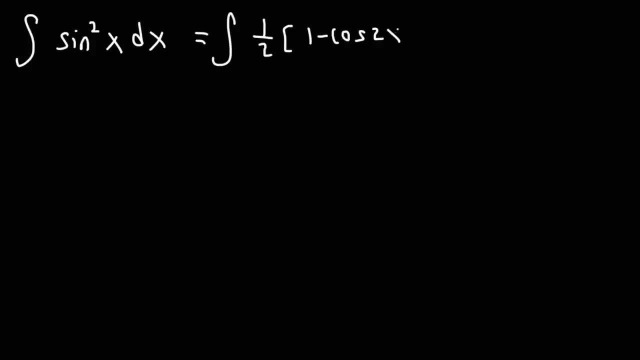 Times 1 minus cosine 2 x. So what we could do is move the 1 half to the front And focus on what we have here. The antiderivative of 1. Is going to be- Let's put this in parentheses. 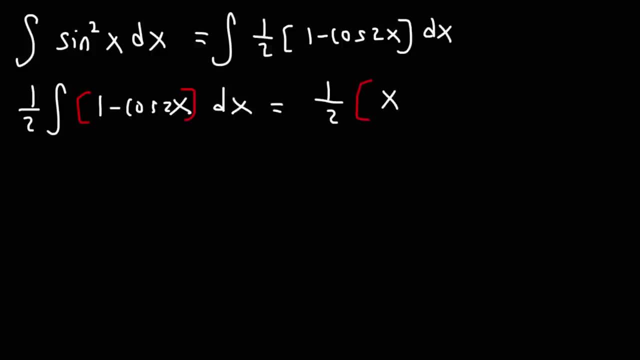 X. Now the antiderivative of cosine 2 x. The antiderivative of cosine Is Sine, But for negative cosine it's going to be negative, sine 2 x. But we need to divide it by the derivative. 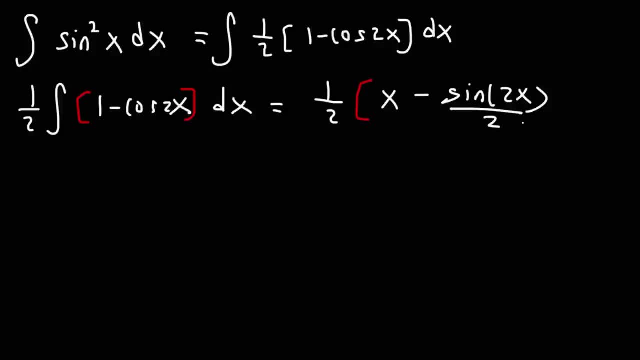 Of the inside. The derivative of 2 x is 2.. So we're going to divide this by 2.. So that's the antiderivative of Negative cosine 2 x. It's negative sine 2 x Divided by 2.. 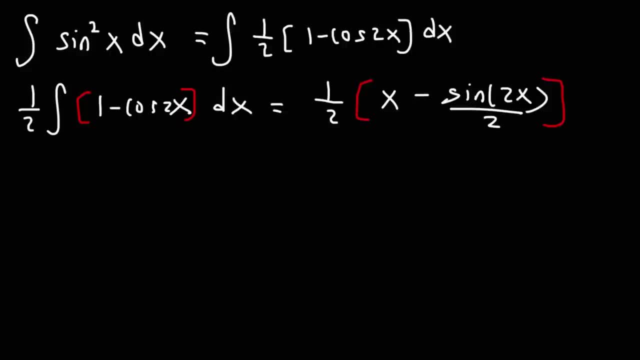 Now all we need to do at this point Is distribute the 1 half. We could leave our answer like this, If you want to, but Let's go ahead and distribute the 1 half, So it's going to be 1 half x. 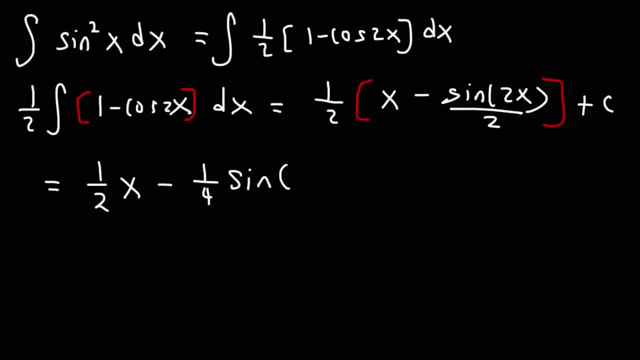 Minus 1. fourth, Sine 2 x plus c. So this is the antiderivative Of sine squared Using A double angle. Now keep in mind We can always Replace sine 2 x With 2 sine x, cosine x. 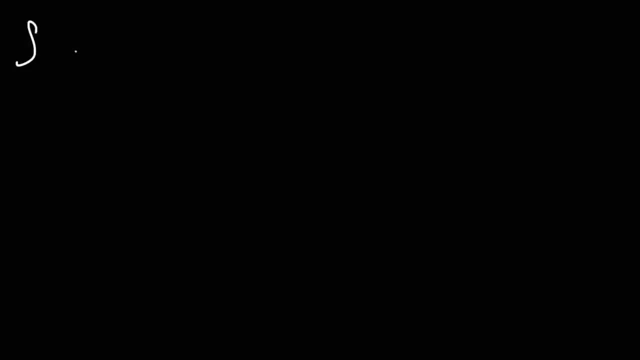 Using the double angle formula. But let's go ahead and move on to the next problem. Let's find the antiderivative of. Instead of cosine squared, Let's make this Cosine squared of 3 x. So go ahead and try that. 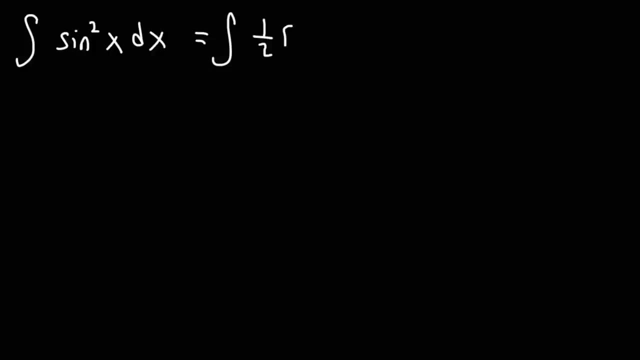 sine squared is 1 half times 1 minus cosine 2x. So what we could do is move the 1 half to the front And focus on what we have here. The antiderivative of 1 is going to be- let's put this in parenthesis- 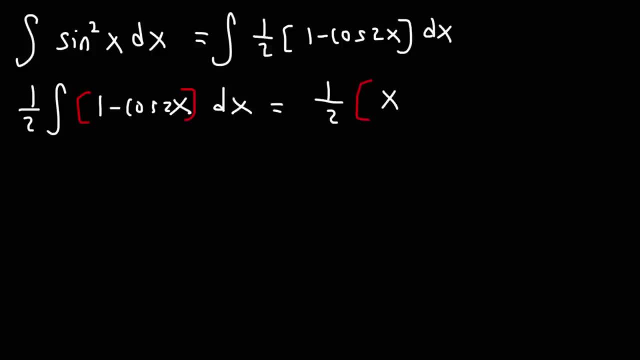 x. Now the antiderivative of cosine, 2x. the antiderivative of cosine is sine, but for negative cosine it's going to be negative sine 2x, but we need to divide it by the derivative of the inside. The derivative of 2x is 2.. 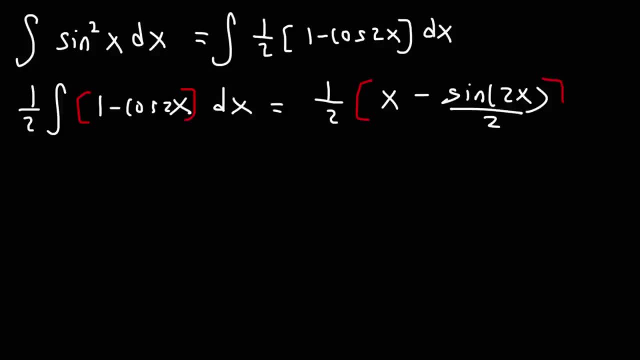 So we're going to divide this by 2.. So that's the antiderivative of negative cosine 2x. It's negative sine 2x divided by 2.. Now all we need to do at this point is distribute the 1 half. 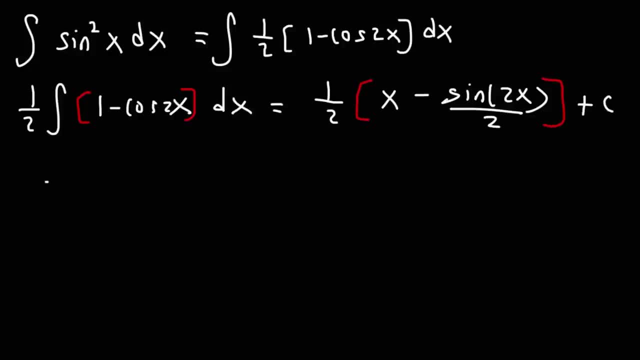 We could leave our answer like this if we want to, but let's go ahead and distribute the 1 half, So it's going to be 1 half x minus 1. fourth sine: 2x plus c. So this is the antiderivative. 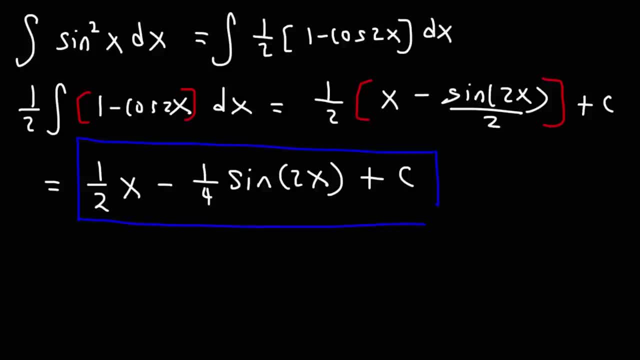 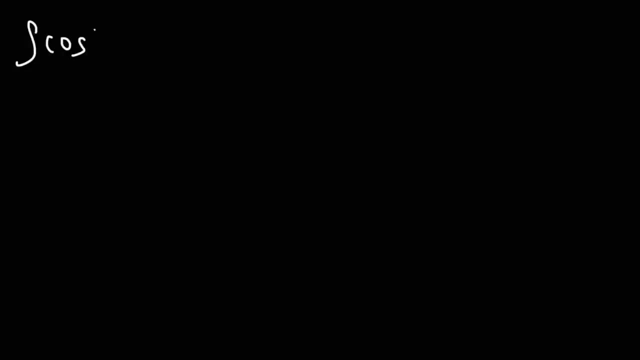 of sine squared using a double angle. Now keep in mind, we can always replace sine 2x with 2, sine x, cosine x, using the double angle formula. But let's go ahead and move on to the next problem. Let's find the antiderivative. 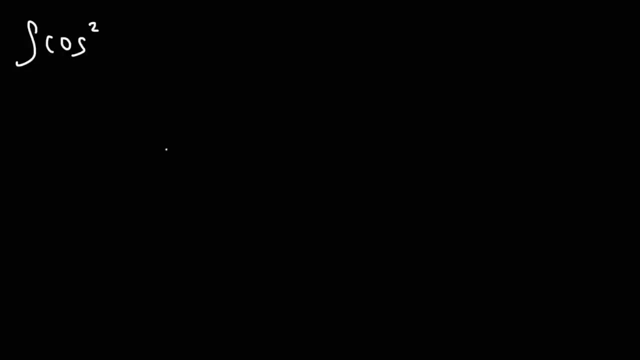 of. instead of cosine squared, let's make this cosine squared of 3x. So go ahead and do that. So go ahead and try that. So first we need to talk about the power reducing formula of cosine squared. Cosine squared x is 1 half. 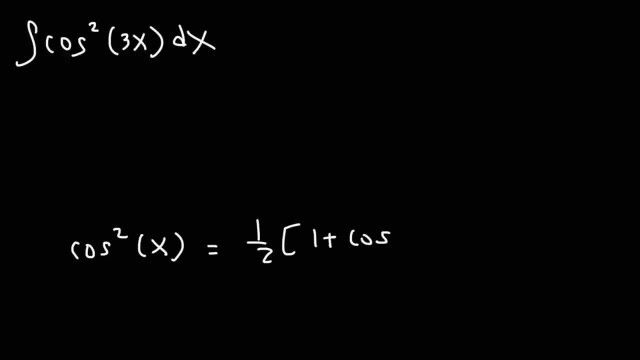 1 plus cosine 2x. So notice the angle. It went from x to 2x, It doubled. What we have here is cosine squared 3x. So using the power reducing formula we can get the cosine squared 3x. 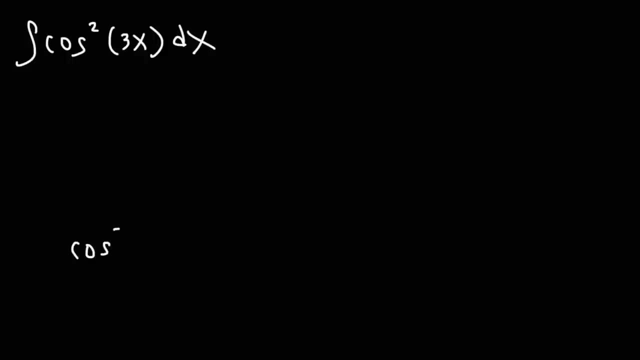 So first we need to talk about The power reducing formula of cosine squared. Cosine squared x Is 1 half 1 plus Cosine 2 x. So notice the angle. It went from x to 2 x. 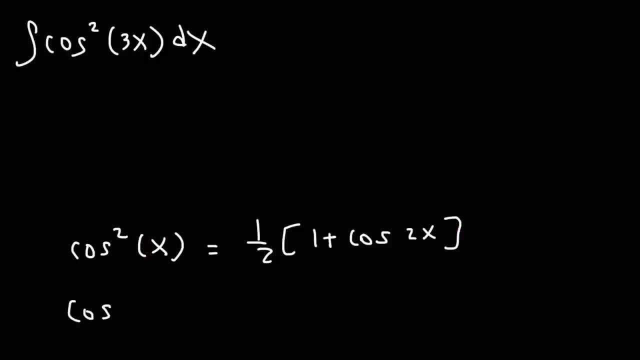 It doubled. What we have here is cosine squared 3 x. So, using the power reducing formula, The angle is going to double. It's going to go from 3 x to 6 x. So this is going to be 1 half. 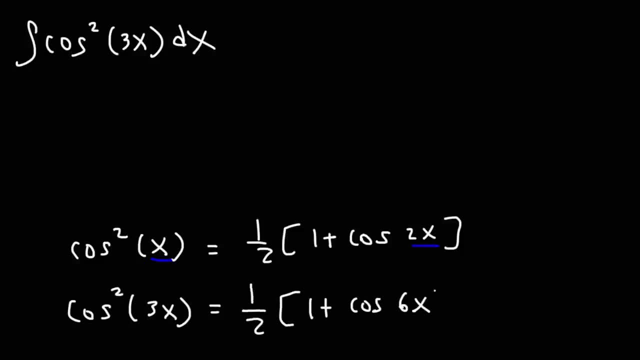 Times 1 plus cosine 6 x. So we're going to have 1 half Integral, 1 plus cosine 6 x And then dx. So now we can find the antiderivative, The antiderivative of 1.. 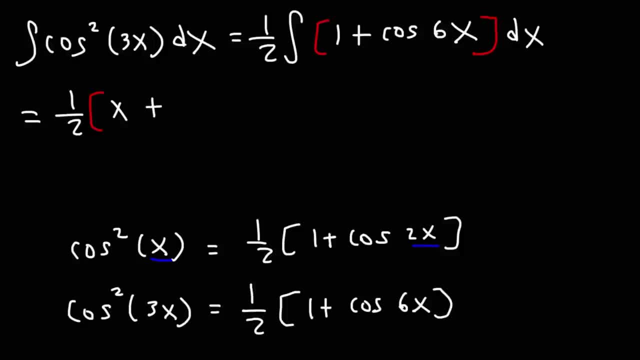 Is going to be x, And the antiderivative of cosine 6 x, That's going to be sine 6 x Divided by the derivative of 6 x, Which is 6.. And, of course, plus c. So now, the last thing that we need to do, 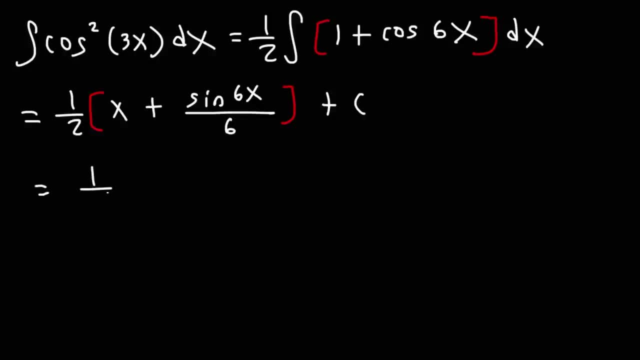 Is: distribute the 1 half. So we're going to have 1 half x Plus 1 over 12.. Sine 6 x plus c. This, right here, is the final answer. Now for the next problem. We're going to try finding the indefinite integral. 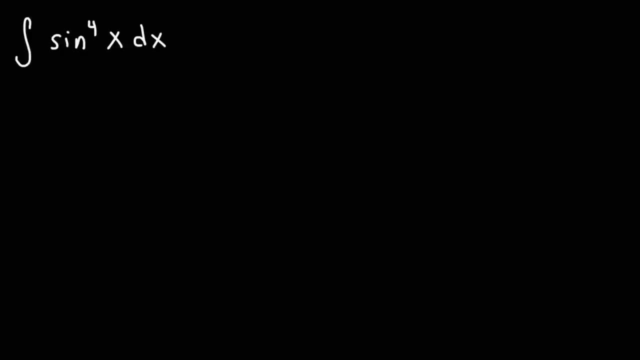 Of sine to the Fourth, x, Dx. So go ahead and try that problem. So this is the integral of Sine squared x, And that Is going to be squared as well. Sine squared raised to the second power Is the same as sine to the fourth. 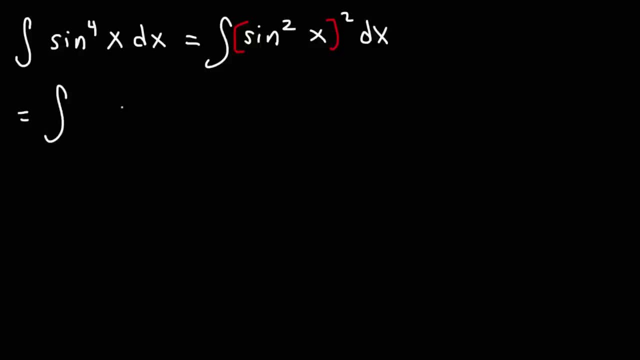 And now we could use The power reducing formula On sine squared. So it's going to be A half Times 1., And then not plus But minus cosine 2x, And then all raised to the second power. 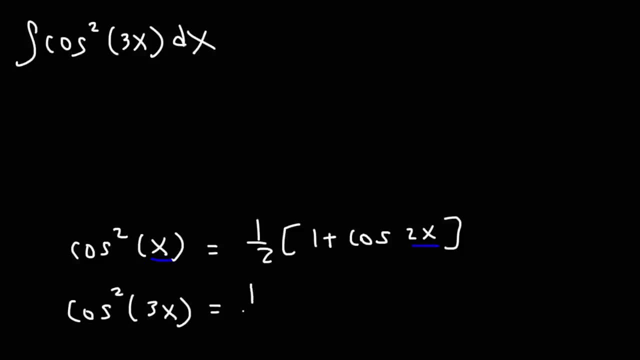 The angle is going to double. It's going to go from 3x to 6x. So this is going to be 1 half times 1 plus cosine 6x. So we're going to have 1 half integral, 1 plus cosine. 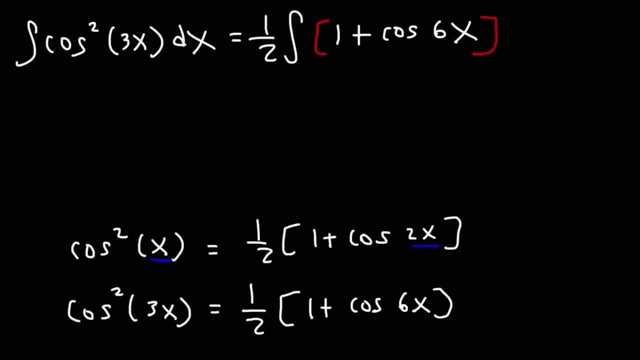 6x and then dx. So now we can find the antiderivative. The antiderivative of 1 is going to be x and the antiderivative of cosine 6x, that's going to be sine 6x divided by the derivative of 6x. 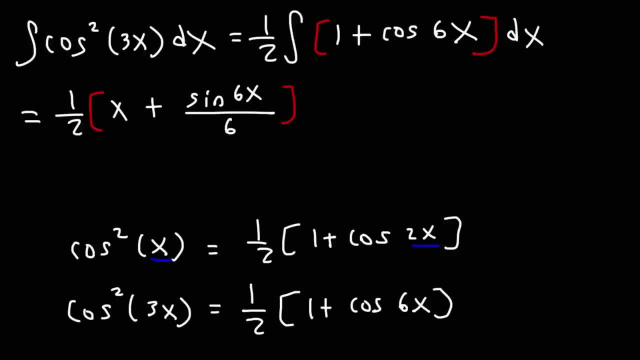 which is 6 and, of course, plus c. So now the last thing that we need to do is distribute the 1 half, So we're going to have 1 half x plus 1 over 12 sine 6x plus c. This, right here, is the final answer. 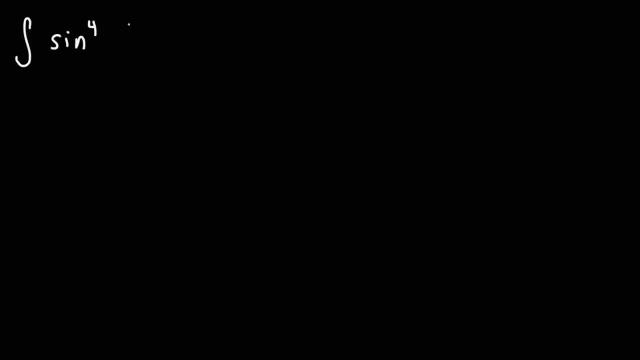 Now for the next problem. we're going to try finding the indefinite integral of sine to the 4th x, dx. So go ahead and try that problem. So this is the integral of sine squared x, and that is going to be squared as well. 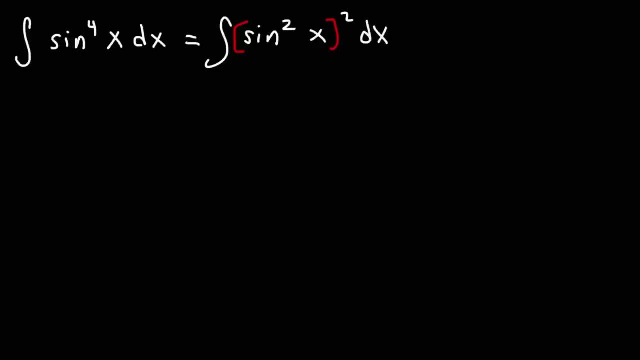 Sine squared raised to the 2nd power is the same as sine to the 4th, And now we could use the power reducing formula on sine squared. So it's going to be a half times 1 and then not plus but minus cosine. 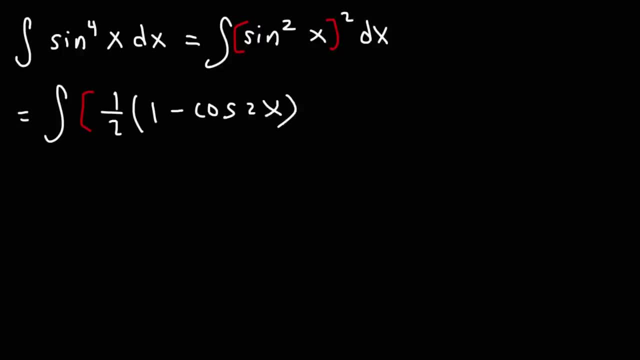 2x and then all raised to the 2nd power. Now we're going to distribute the exponent. So if we distribute 2x to 1 half it's going to be 1 half squared, so that becomes 1: 4th. 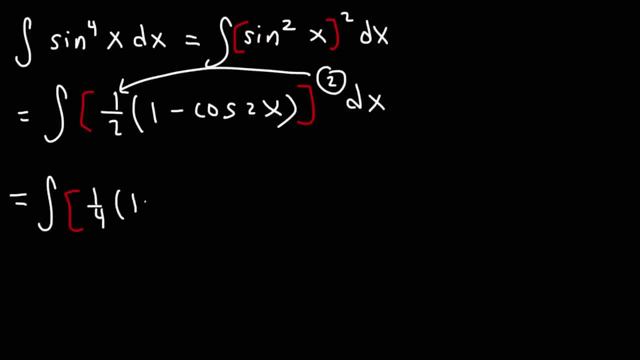 and then we're going to have 1 minus cosine 2x raised to the 2nd power, which means we need to FOIL that Now we can move the 1, 4th to the front, So we have 1 over 4. 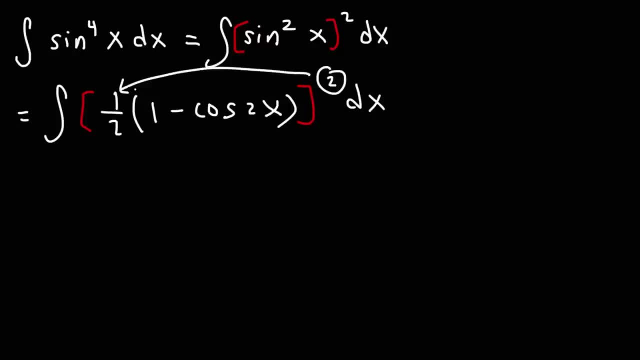 Now we're going to distribute the exponent. So if we distribute to 1 half, it's going to be 1 half squared, So that becomes 1 fourth. And then we're going to have 1 minus cosine 2x. 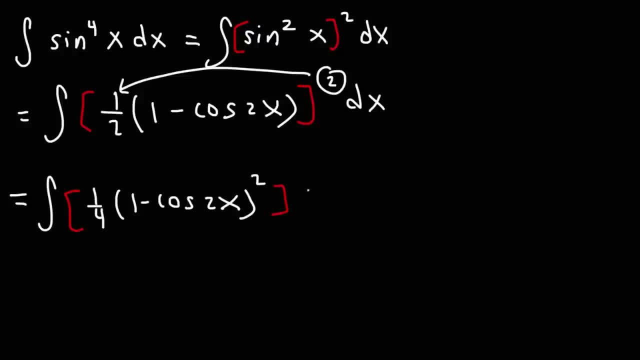 Raised to the second power, Which means we need to FOIL that. Now we can move the 1 fourth to the front, So we have 1 over 4.. Integral: 1 minus cosine: 2x Times 1 minus cosine. 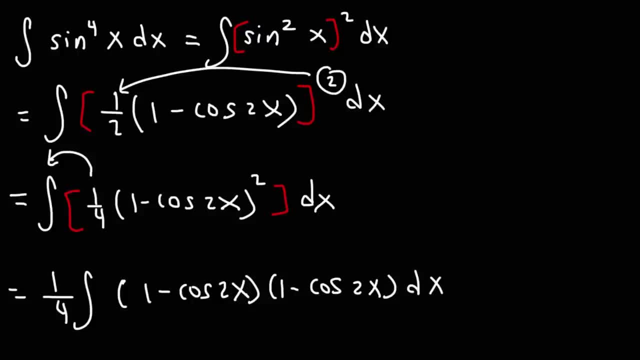 2x, dx, x. So first we have 1 times 1, which is 1.. And then this is going to be negative cosine 2x plus another negative cosine 2x, that's negative 2 cosine 2x, and then negative cosine 2x times negative cosine 2x, that's positive cosine squared of 2x. 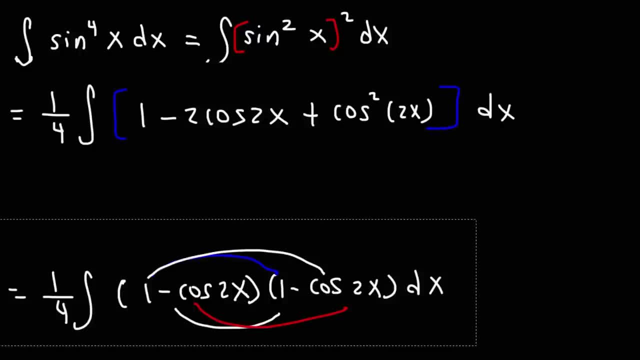 Now, before we integrate this expression, Let's use the power reducing formula on cosine squared 2x. So we know cosine squared of 1x Is 1 half 1 plus Cosine 2x, So therefore, cosine squared of 2x. 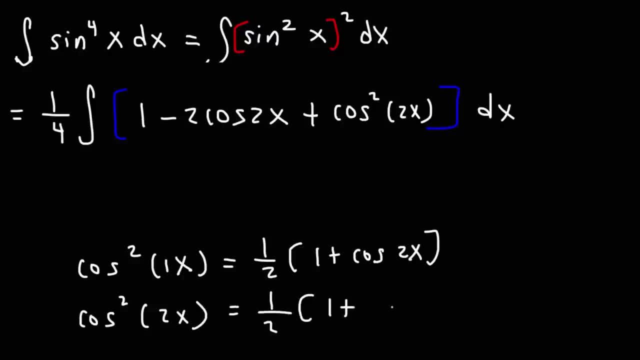 Is going to be 1 half 1 plus Cosine 4x. So the key, The key here is to realize that when you're using the power reducing formula, the angle doubles. so if it doubles from 1x to 2x, then if we start from 2x it's going to double to 4x. 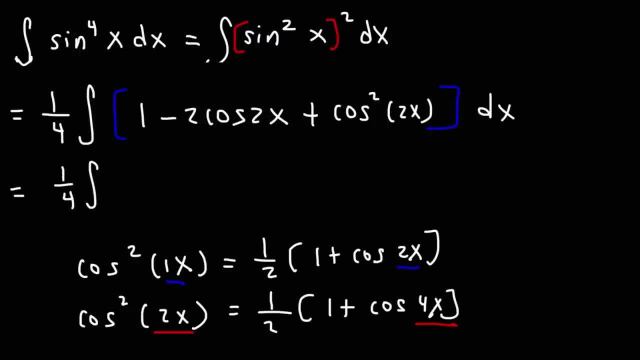 So this becomes 1 fourth integral, 1 minus 2 cosine 2x, And then plus 1 half. Well, let's distribute the half. So this is 1 half times 1, or just 1 half, And then this is going to be plus. 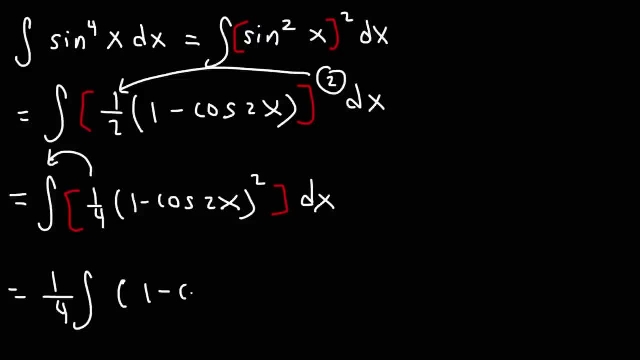 integral: 1 minus cosine 2x times 1 minus cosine 2x d x. So first we have 1 times 1, which is 1, and then this is going to be negative cosine 2x plus another negative cosine 2x. 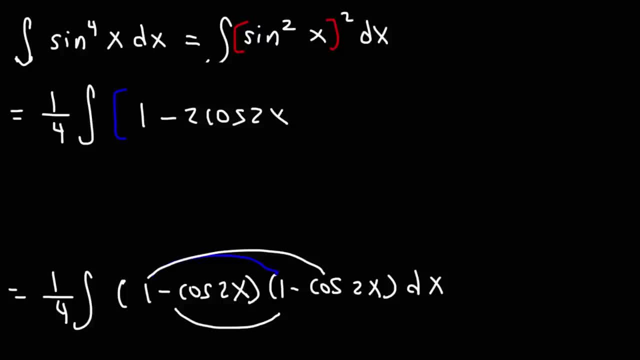 that's negative 2 cosine 2x. and then we're going to have negative cosine 2x times negative cosine 2x, that's positive cosine squared of 2x. Now, before we integrate this expression, let's use the power reducing formula on. 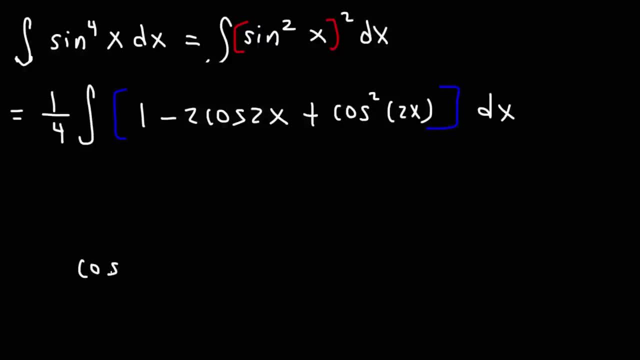 cosine squared 2x. So we know cosine squared of 1x is 1 half 1 plus cosine 2x. so therefore cosine squared of 2x is going to be 1 half 1 plus cosine 4x. so the key here is to realize that. 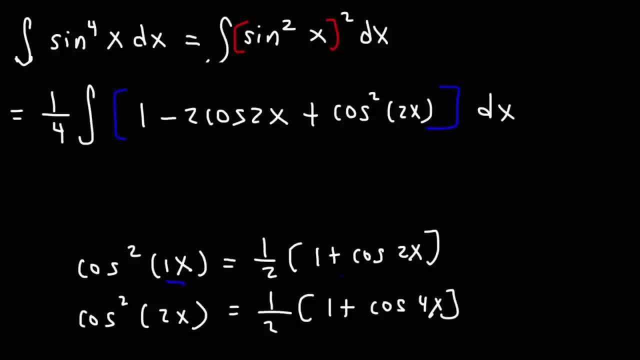 when you're using the power reducing formula, the angle doubles. so if it doubles from 1x to 2x, then if we start from 2x it's going to double to 4x. So this becomes 1, 4th integral of 2x. 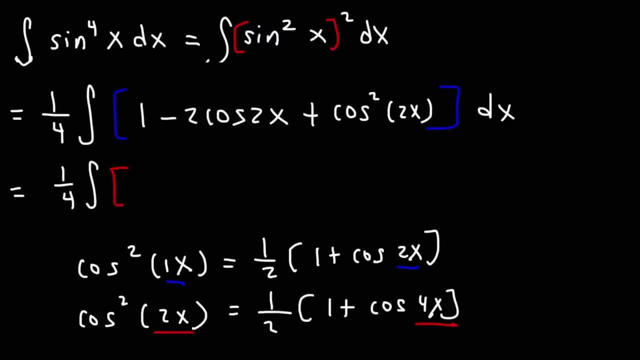 So this becomes 1 4th integral of 2x. So told us that if we take the cosine 2x times 1 x, that'säch we would have Al kommen 0 aqui in this broken down equation. So 1 half of cosine 2x. 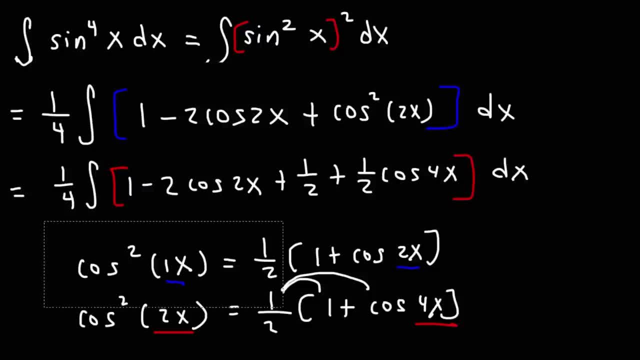 plus 1 half of cosine 2x. Well, let's distribute to half, Okay, So this is 1 half times 1, or just 1 half, And then this is going to be plus 1 half cosine 4x. 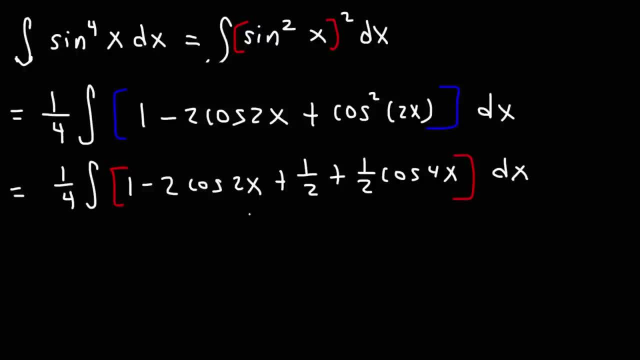 Now what we could do is combine like terms: 1 plus 1, half 1 is 2 over 2, so plus 1 over 2, that becomes 3 over 2.. So we can just put 3 over 2 here. 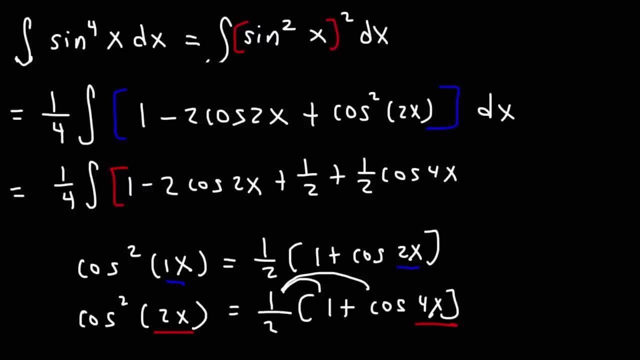 1 half Cosine 4x. Now what we could do is combine like terms: 1 plus 1 half 1 is 2 over 2.. So plus 1 over 2, that becomes 3 over 2.. 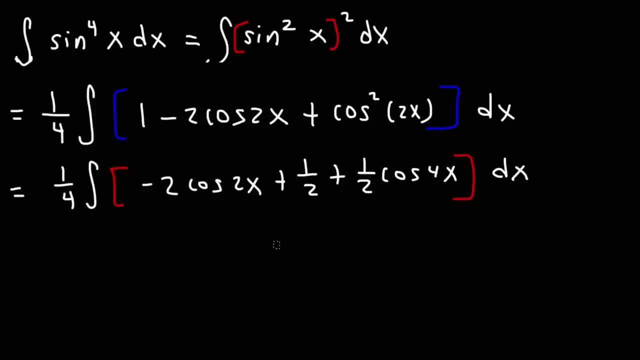 So we can just put 3 over 2 here. And now let's find the antiderivative. So the antiderivative of negative 2, cosine 2x, That's going to be negative 2.. The antiderivative of cosine is negative sine. 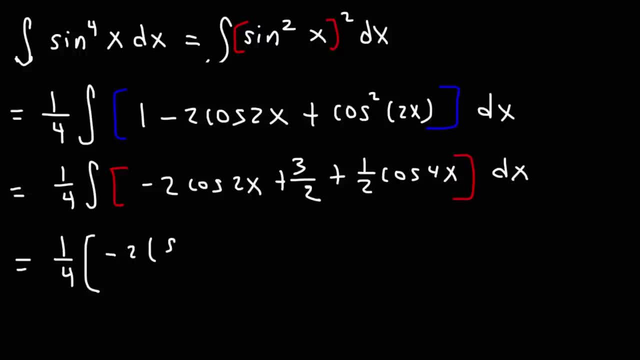 I mean not negative sine, but positive sine: 2x, 2x Divided by 2.. The antiderivative of 3 over 2 is just 3 over 2 times x, And for cosine to the 4x is going to be sine to the 4x over 4.. 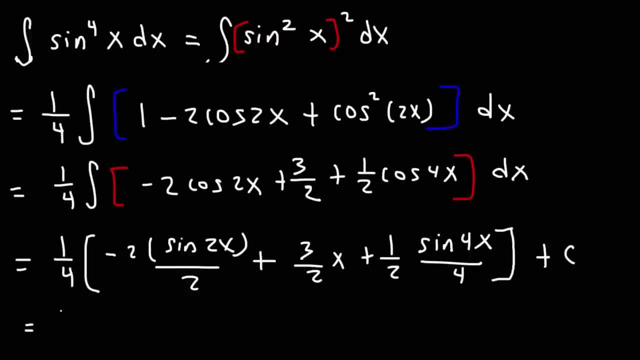 And then, of course, plus c. Now let's organize our answer. So I'm going to keep the 1 fourth in the front. I'm going to write this one first. So plus or just 3 over 2x. Now these 2's will cancel. 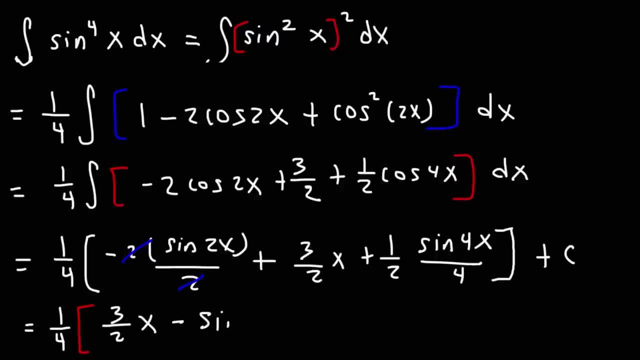 So we're just going to write this one first. So we're just going to have minus sine 2x, And this is going to be 1 over 8 sine 4x, And then plus the constant of integration. So this is the antiderivative of sine to the 4th x. 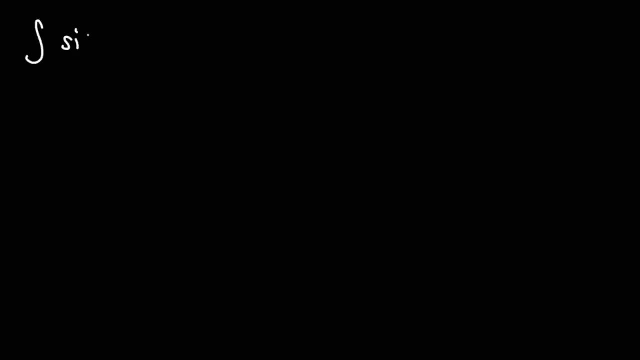 Now let's try this problem. What is the antiderivative of sine squared, cosine squared, dx? Go ahead and try that. So for this problem we need to use the power reducing formulas on sine squared and cosine squared. So sine squared is 1, half times 1, minus cosine 2x. 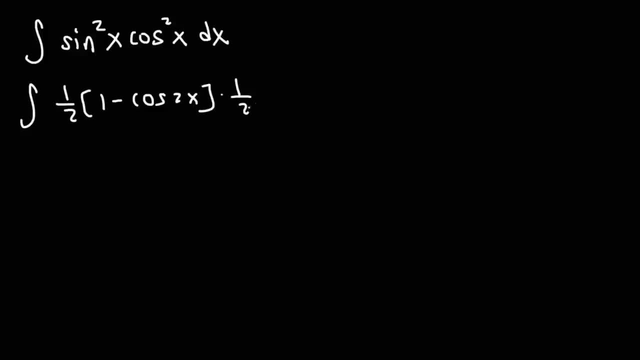 Cosine squared is 1 half, But 1 plus Cosine squared is 1 half times 1 minus cosine 2x. 1 half times 1 half is 1 over 4. So we can move that to the front. 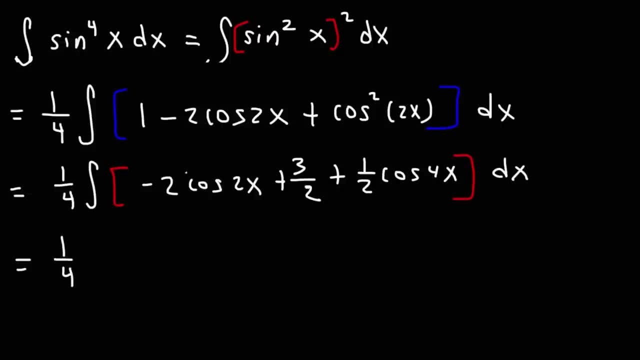 And now let's find the antiderivative. So the antiderivative of negative 2, cosine 2x, that's going to be negative 2.. The antiderivative of cosine is negative sine. I mean not negative sine, but positive sine. 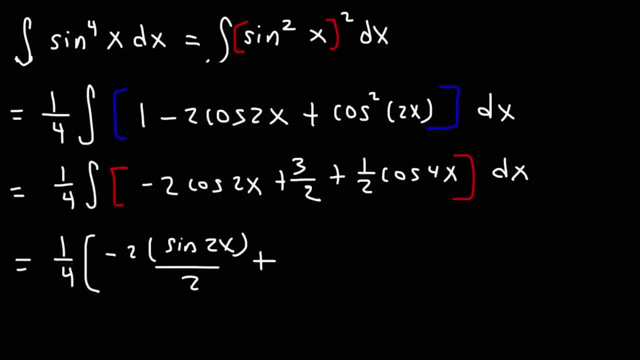 2x divided by 2.. The antiderivative of 3 over 2 is just 3 over 2 times x, And for cosine to the 4x, it's going to be sine to the 4x over 4.. 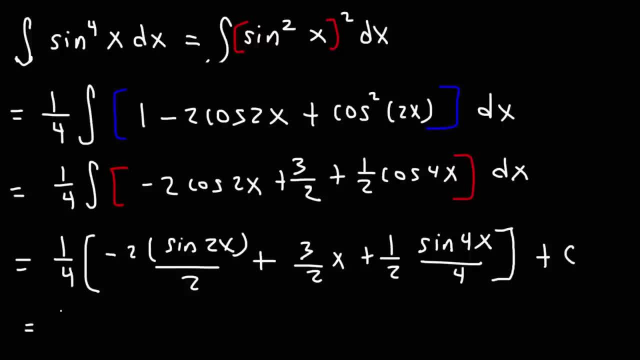 And then, of course, plus c. Now let's organize our answer. So I'm going to keep the 1 fourth in the front. I'm going to write this one first. So plus or just 3 over 2x. 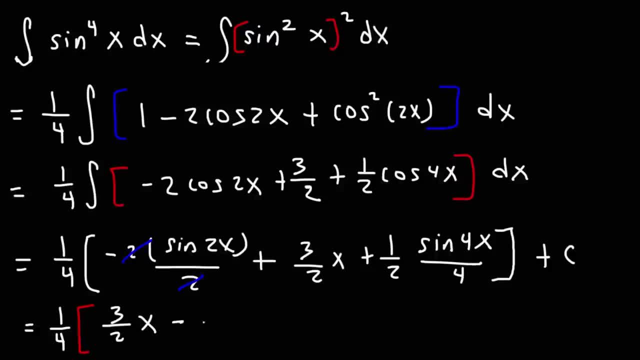 Now these 2s will cancel. so we're just going to have minus sine 2x And this is going to be 1 over 8 sine 4x And then plus the constant of integration. So this is the antiderivative of sine to the 4th x. 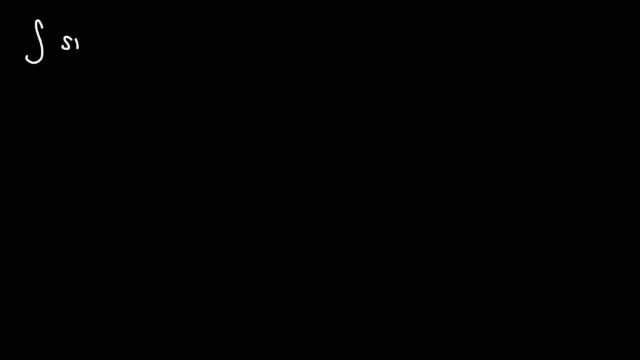 Now let's try this problem. What is the antiderivative of sine squared, cosine squared, dx? Go ahead and try that. So for this problem we need to use the power of 2. And we're going to reduce in formulas on sine squared and cosine squared. 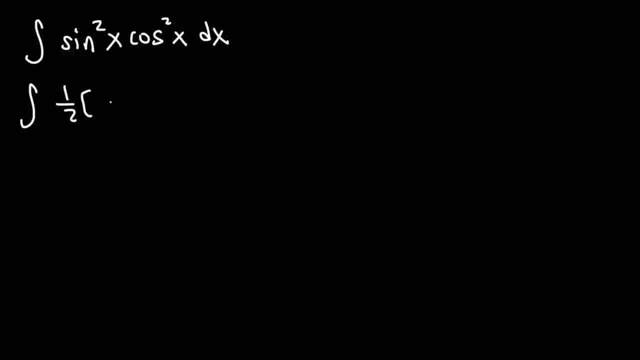 So sine squared is 1 half times 1 minus cosine 2x Cosine squared is 1 half, but 1 plus cosine 2x 1 half times 1 half is 1 over 4.. So we can move that to the front. 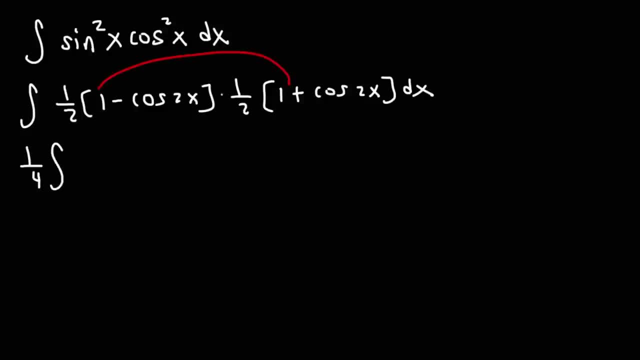 And then we need to FOIL. So here we have: We have 1 times 1.. So that's going to be 1.. And then positive cosine 2x will cancel with negative cosine 2x, So the 2 middle terms cancel. 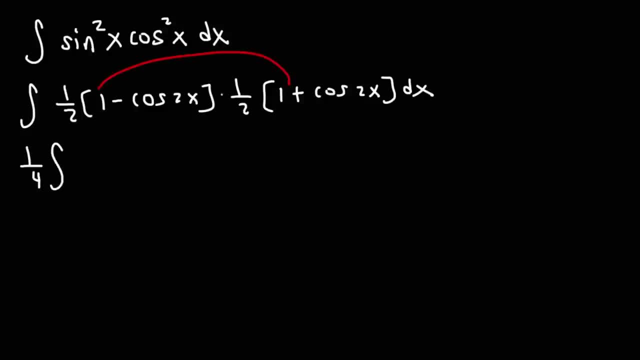 And then we need to FOIL. So here we have 1 times 1.. So that's going to be 1.. And then positive cosine 2x will cancel with negative cosine 2x, So the 2 middle terms cancel. 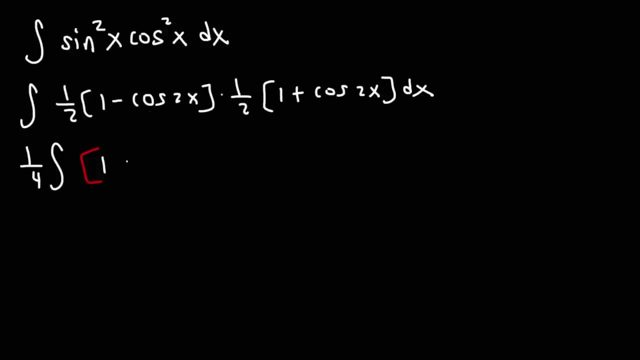 And then negative cosine times. positive cosine is going to give us Negative cosine squared of 2x 1 minus cosine squared. That's an identity. 1 minus cosine squared is equal to sine squared. So what we now have is 1 fourth integral sine squared: 2x- dx. 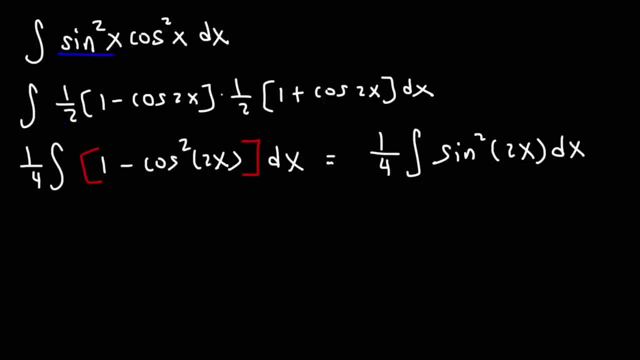 Now, if sine squared 1x is this, Sine squared 2x must be the same thing, but with a 4x here Instead of a 2x. So what we now have is 1 fourth integral And then using the power reducing formula. 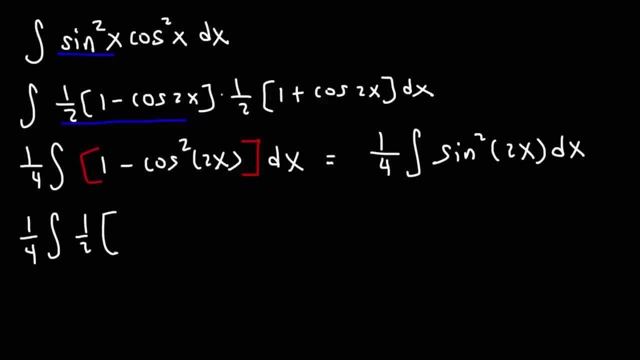 This is going to be 1 half times 1 minus cosine, But not 2x. This is going to double to 4x. Now 1 fourth and 1 half we can combine, So it's 1 over 8 integral. 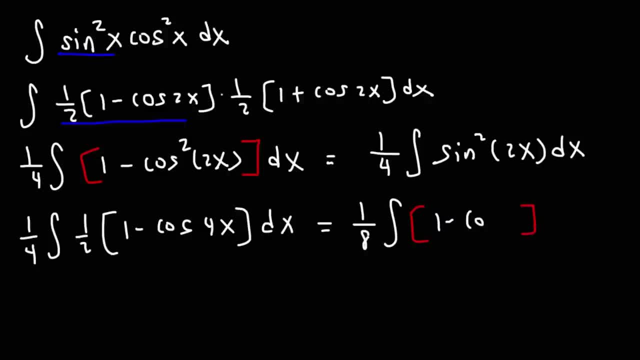 1 minus cosine, 4x, dx. The antiderivative of 1 is x, The antiderivative of cosine is going to be sine, But 4x divided by the derivative of 4x, which is 4.. And then plus c. 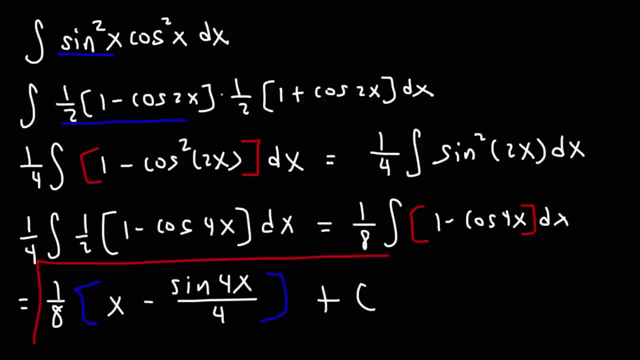 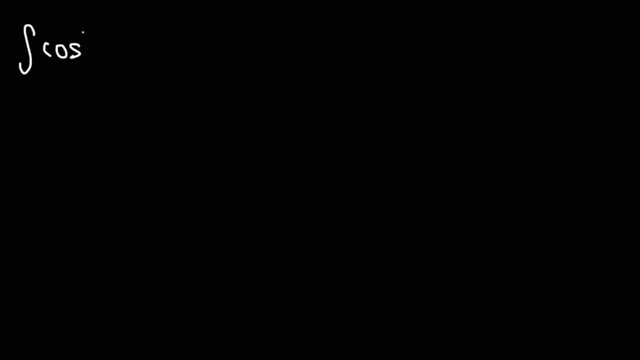 So this is the final answer to the problem. For the next problem, we're going to find the indefinite integral of cosine squared times tangent to the third power. So what do you think we need to do here in order to find the indefinite integral of this expression? 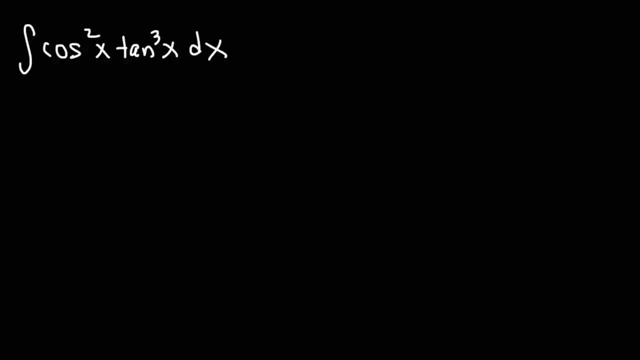 Well, we don't know of an identity that involves cosine and tangent, So the best thing to do is to find the indefinite integral of this expression. So what we need to do is to convert tangent into sine over cosine. So tangent cube is going to be sine to the third, divided by cosine cube. 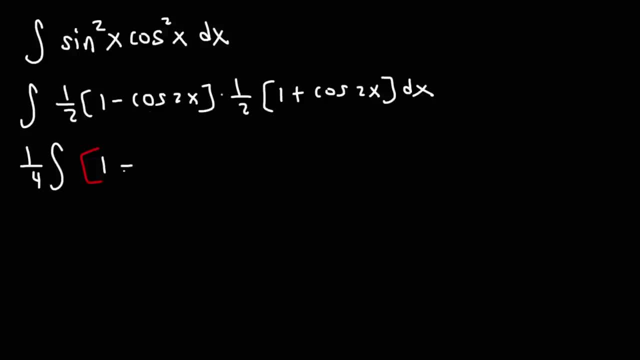 And then negative cosine times positive cosine is going to give us negative cosine squared of 2x 1 minus cosine squared. that's an identity. 1 minus cosine squared is equal to sine squared. So what we now have is 1 fourth integral sine squared: 2x dx. 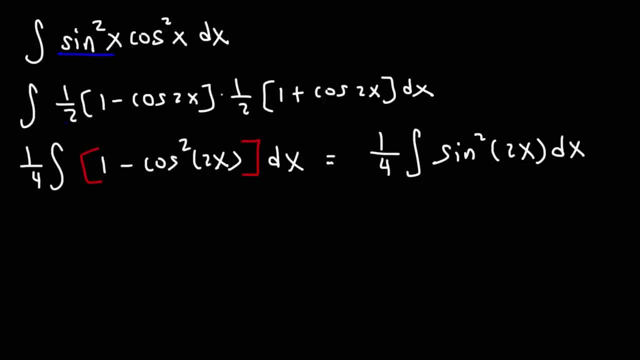 Now, if sine squared 1x is this, sine squared 2x must be the same thing, but with a 4x here instead of a 2x. So what we now have is 1, fourth integral And then using the power reducing formula. 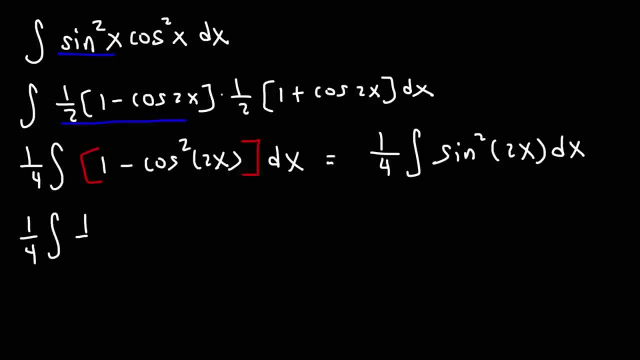 this is going to be 1 half, 1 half times 1 minus cosine, but not 2x. this is going to double to 4x. Now 1 fourth and 1 half we can combine, So it's 1 over 8 integral. 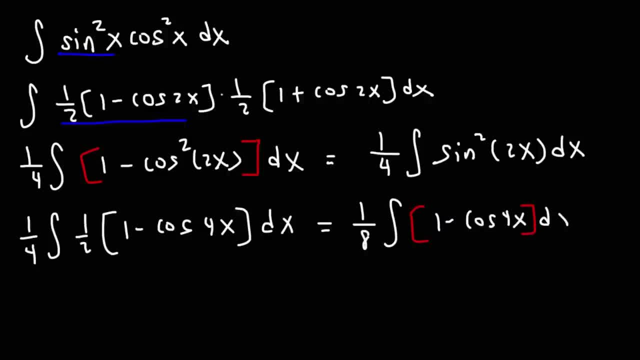 1 minus cosine, 4x, dx. The antiderivative of 1 is x, The antiderivative of cosine is going to be sine, but 4x divided by the derivative of 4x, which is 4.. And then plus c. 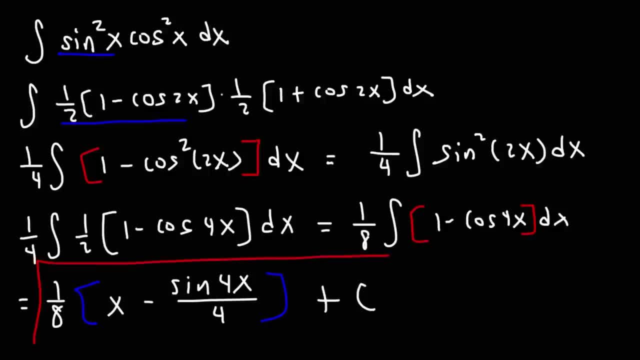 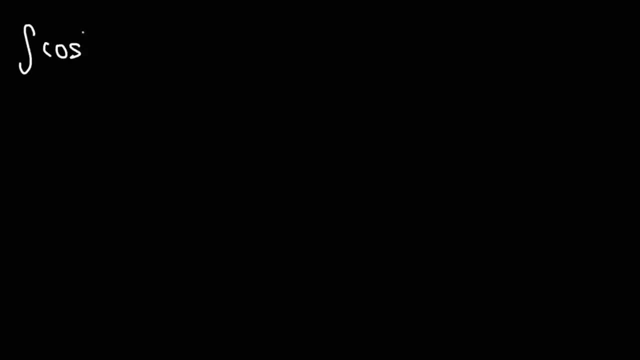 So this is the final answer to the problem. For the next problem, we're going to find the indefinite integral of cosine squared. So what do you think we need to do here in order to find the indefinite integral of this expression? Well, we don't know of an identity that involves cosine and tangent. 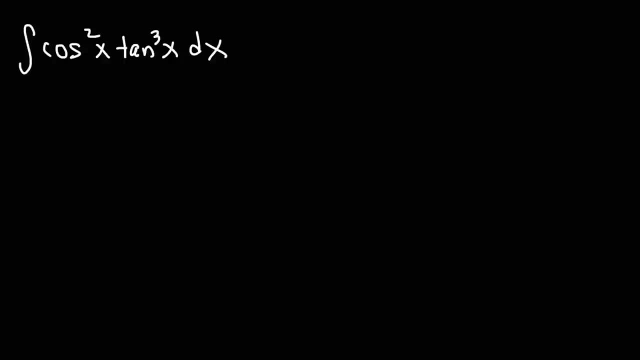 So the best thing to do is to convert tangent into sine over cosine. So tangent cubed is going to be sine to the third divided by cosine cubed. Or we could write cosine cubed as cosine squared times cosine. So that way we can easily cancel out a cosine squared. 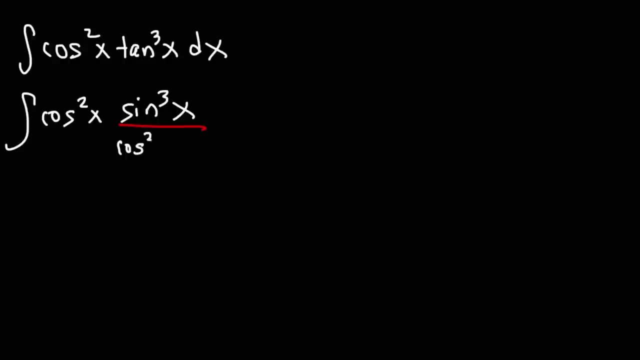 Or we can write cosine cube as cosine squared times cosine, So that way we can easily cancel out a cosine squared. Now, if we try to make u equal to sine, du is going to be cosine dx. But the cosine is on the bottom, not on the top still. 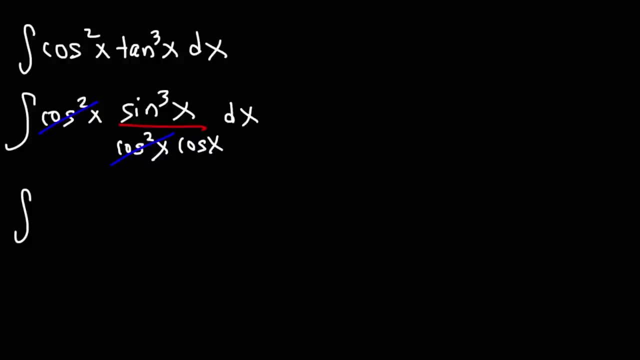 It's not going to cancel well the way it is. So we want to make u equal to sine. I mean u equal to cosine, not sine. So what we're going to do is we're going to split up sine cube into sine squared. 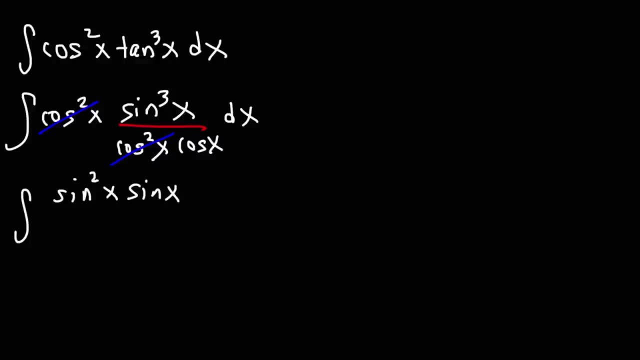 Times sine, And we'll leave cosine on the bottom for now. Now, in the next step, we're going to change sine squared into 1 minus cosine squared. Now, at this point we can make u equal to cosine x. du is going to be negative sine x dx, and so dx is going to be du over negative sine x. 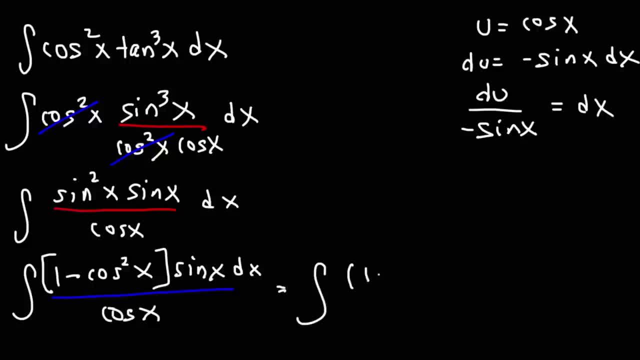 So this becomes 1 minus u squared divided by u, and then we have sine x times du over negative sine. So we can cross that out. and then let's move the negative sine to the front, So we have negative integral. Let's break this up into two smaller fractions, So it's going. 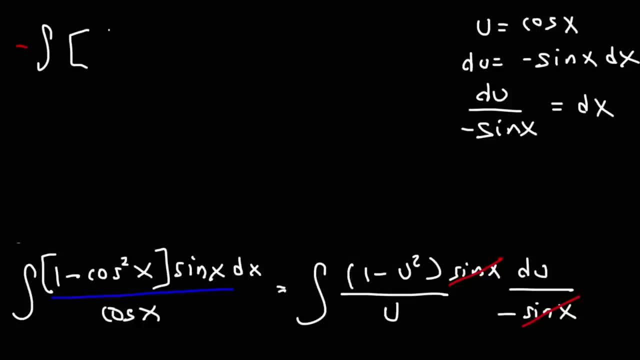 to be 1 over u and then minus u squared over u, which is negative u. So this is going to equal negative ln u and then these two negative signs, they all cancel. So that's going to be positive and the antiderivative of u is going to be u squared. 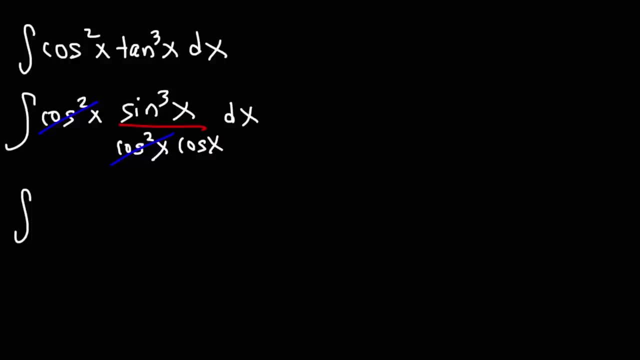 Now, if we try to make u equal to sine, du is going to be cosine dx, But the cosine is on the bottom, not on the top, so it's not going to cancel well the way it is. So we want to make u equal to sine. 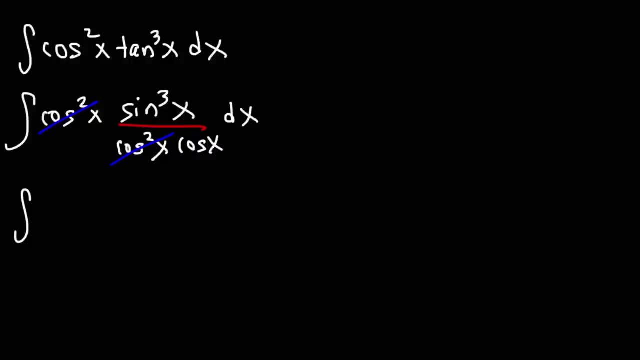 I mean u equal to cosine, not sine. So what we're going to do is we're going to split up sine cubed into sine, squared times sine, And we'll leave cosine on the bottom for now. Now, in the next step, 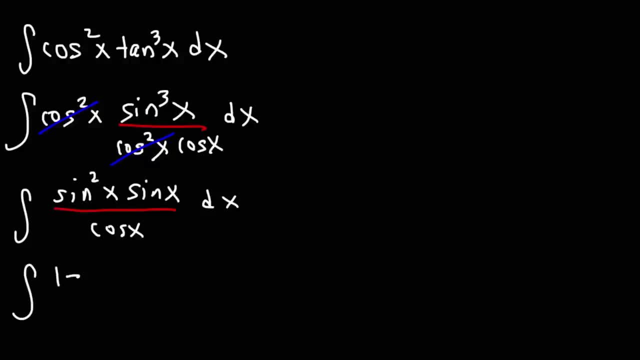 we're going to change sine squared into 1 minus cosine squared. Now at this point we can make u equal to cosine x. du is going to be negative sine x, dx, And so dx is going to be du over negative sine x. 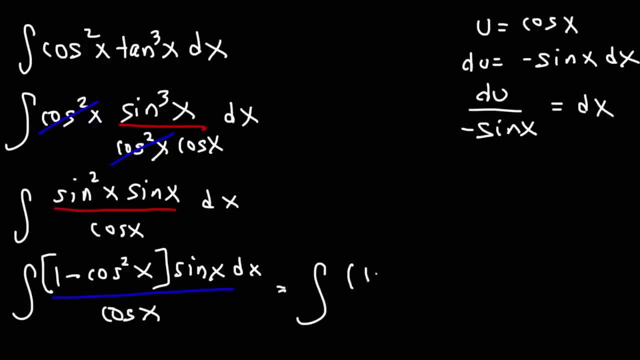 So this becomes 1 minus u squared, divided by u, And then we have sine x times du over negative sine. So we can cross that out. And then let's move the negative sine to the front, So we have negative integral. 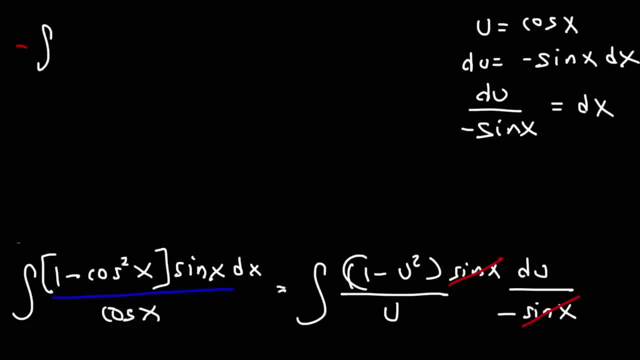 Let's break this up into two smaller fractions, So it's going to be 1 over u And then minus u squared over u, which is negative u. So this is going to equal negative ln u, and then these two negative signs, they all cancel. 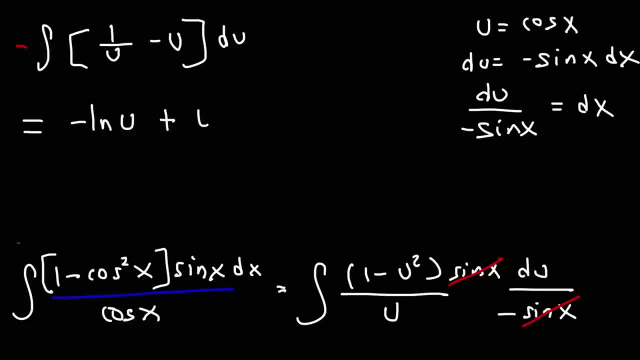 So that's going to be positive, And the antiderivative of u is going to be u squared over 2, plus c. So this is going to be negative ln. and then absolute value: cosine x plus 1, half cosine squared x.